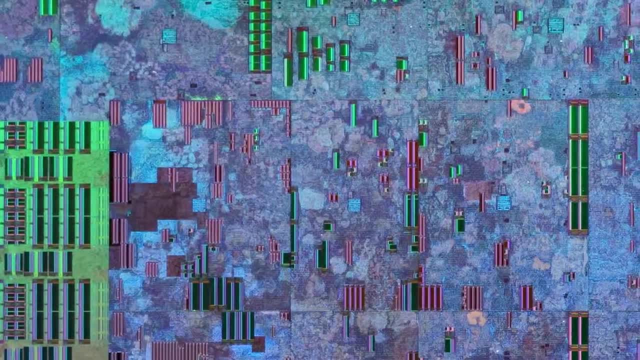 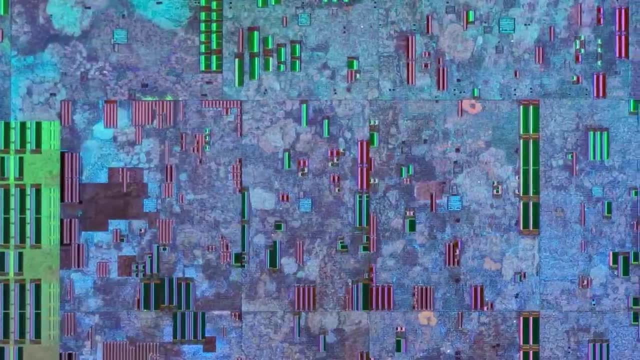 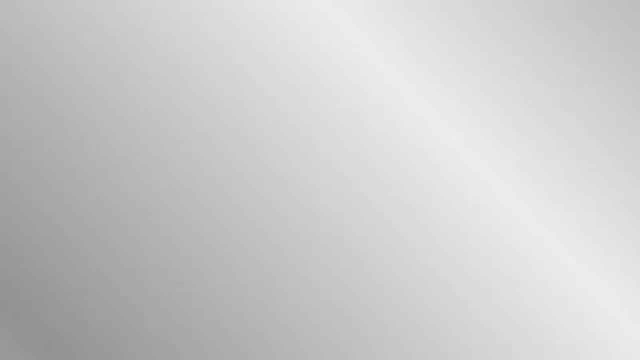 is a warning that I am making massive oversimplifications, which I'm sure you'll point out to me in the comments. That was the warning for the entire video. Modern computers, at their core are electrical circuits. A very simple circuit might consist. 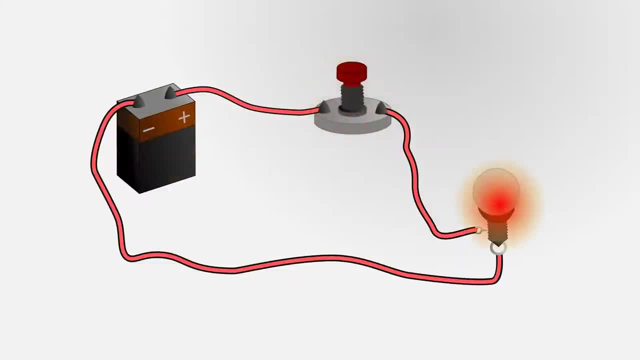 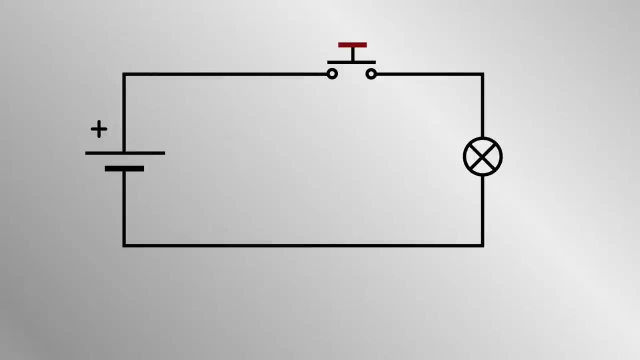 of a battery connected to a switch, then a light bulb, then back to the negative terminal of the battery. Modern computer components typically supply a voltage of 3.3 or 5 volts between the positive terminal and the ground, or negative terminal, if you like to think. 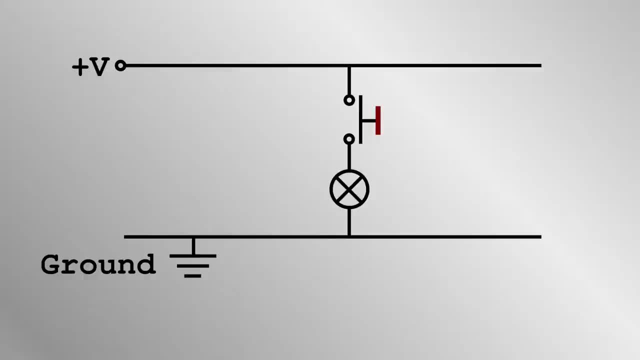 of it. that way, Computers treat information as binary, on or off, true or false, one or zero, Based on if the voltage is high or low. The important component in our circuit here is the push switch, which comes in two flavours: Push to make, that's when a person presses. 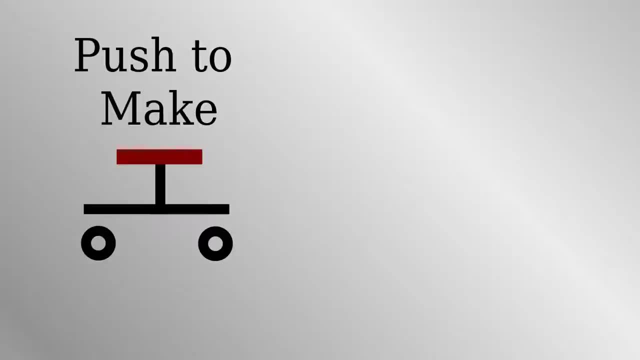 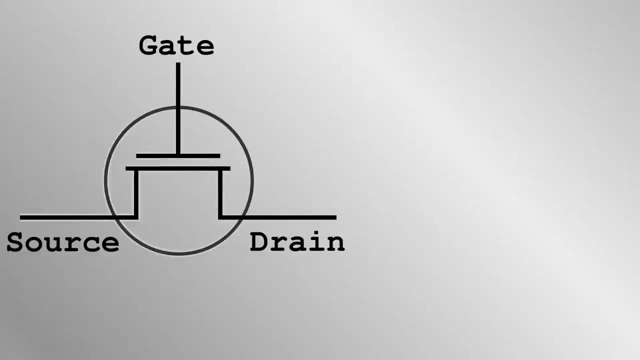 down and the circuit is completed between the two terminals and the bulb lights up. The push to break switch is exactly the opposite. This is the symbol for a transistor. More specifically, it's a metal oxide semiconductor field effect transistor, or MOSFET. It's source. 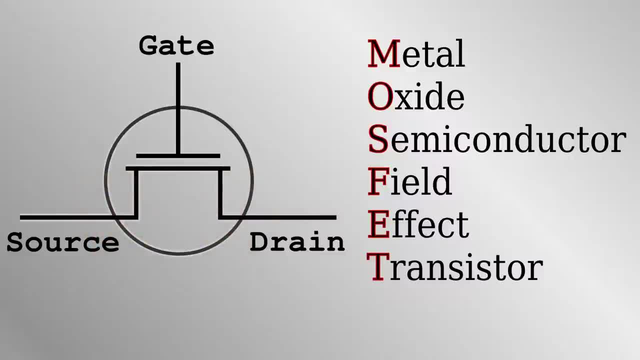 ion, like the two terminals of a switch, But it has a third terminal called a gate. Just like switches there are two types. The n-channel type makes a circuit. when that high voltage is applied to the gate, like a push to make The p-channel breaks the circuit. 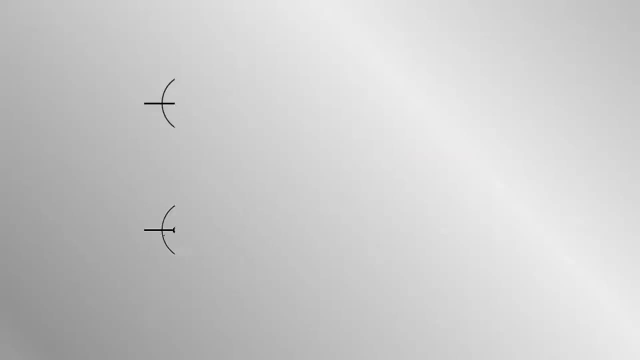 when a high voltage is applied like a push to break, So transistors act like switches, except instead of a person pressing it down, a voltage is applied In modern computers. these types of transistors are used in pairs referred to as CMOS, which 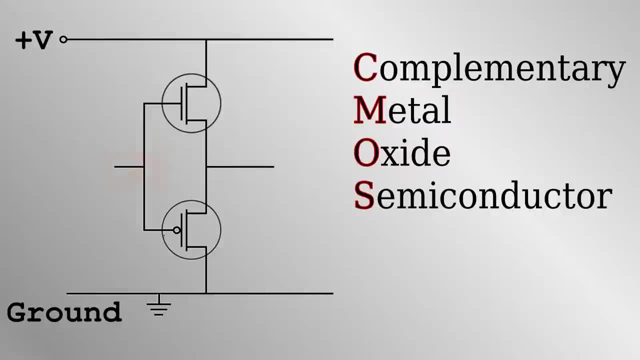 are complementary metal oxide semiconductors. The gate terminals of a given pair are always connected together, so they receive the same input. Here is a simple example. If we apply a high voltage- or 1,- to the input, the n-channel MOSFET opens a route between high voltage. 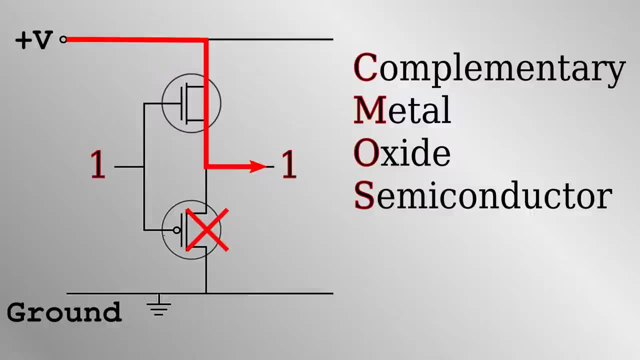 and the output. The p-channel closes the route to ground. If we apply a low voltage- or 0, at the input, the p-channel opens a path to ground. I think it seems pointless. We got the same thing at the output as we did at the input. 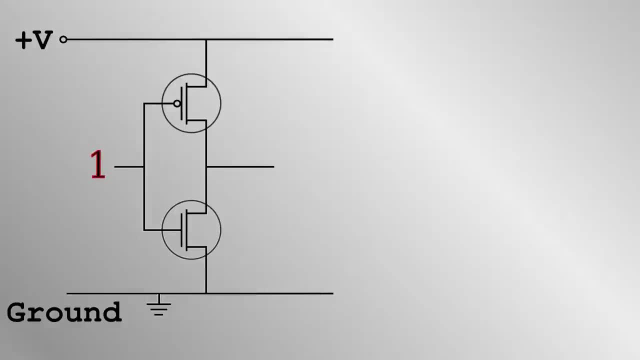 But let's swap around the two MOSFETs. Now, when we apply a high voltage- or 1, to the input, the n-type opens a route to low voltage or 0.. When we apply a 0 to the input, we get: 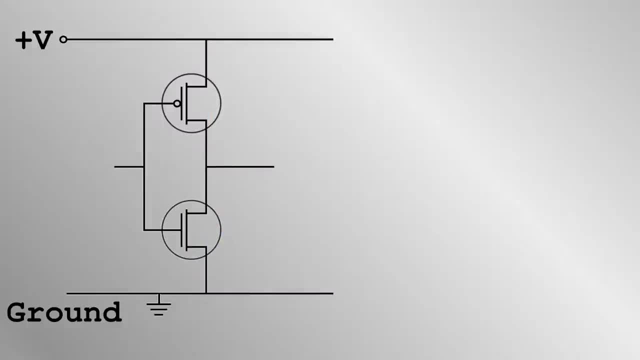 a 1 at the output. Whatever we put in at the input, we get the opposite at the output. Later we will come back to how this forms the basis of all modern processors. Understand that it is vast network of different types of transistors and that there are many different. 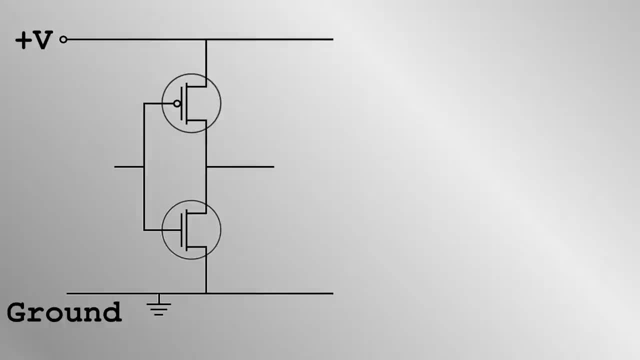 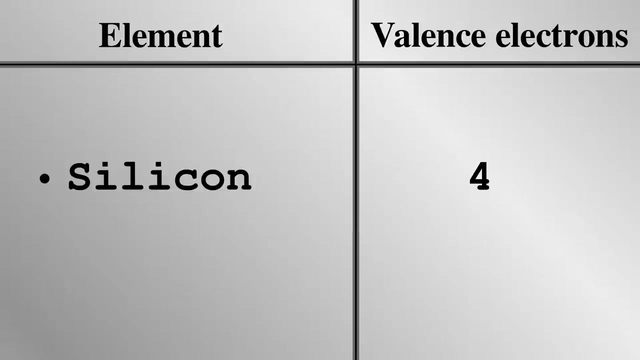 networks of CMOS pairs like these, which allow computers to think. For now, let's see how transistor networks are made in basic terms. Silicon is a semiconductor with four valence electrons which is doped or mixed with other elements. Gallium, for example, has three valence electrons, one less than silicon. 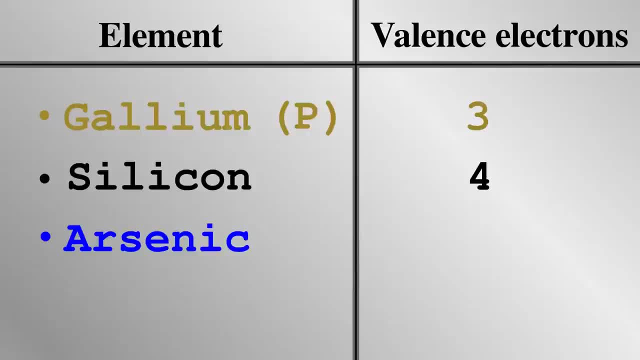 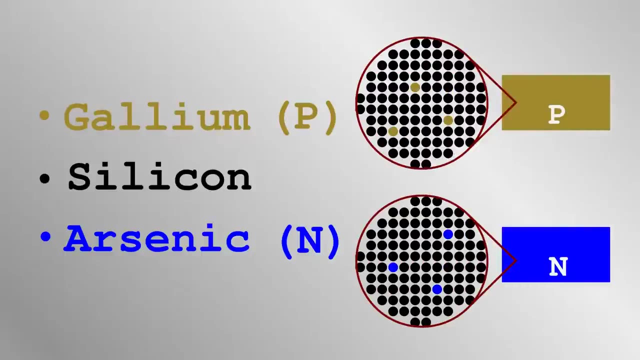 hence more positive or p-type. Meanwhile, an element like arsenic has five valence electrons, one more than silicon, Therefore adding a negative charge, hence n-type Trace amounts of these elements, typically one for every million silicon atoms or so, are implanted by chemical diffusion or by 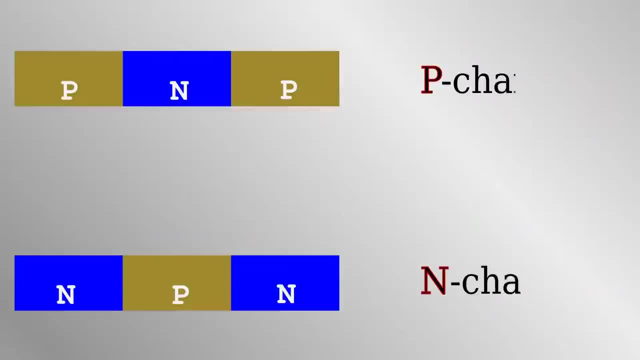 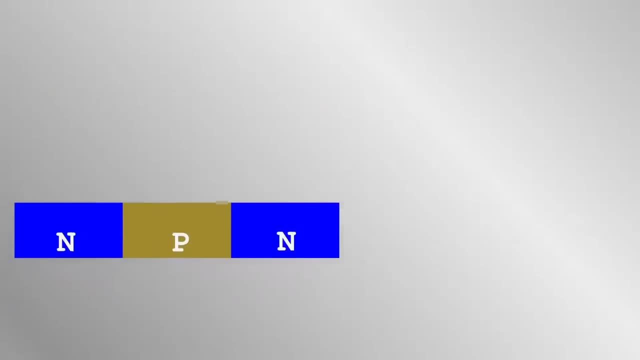 firing them out of a particle accelerator. Transistors are made by sandwiching a region of one of the dopants between two of the other. Let's look more closely at the n-channel configuration. This by itself does not conduct electricity, but when an electric field is, 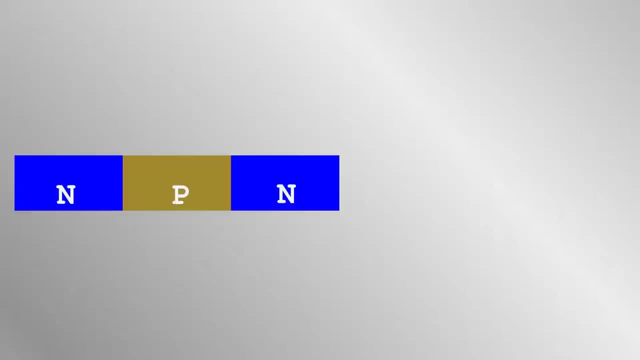 applied to it, a conducting channel forms. This is the n-channel configuration. This is the n-channel configuration. This by itself does not conduct electricity, but when an electric field is applied to it, a conducting channel forms. Hence the name field effect. 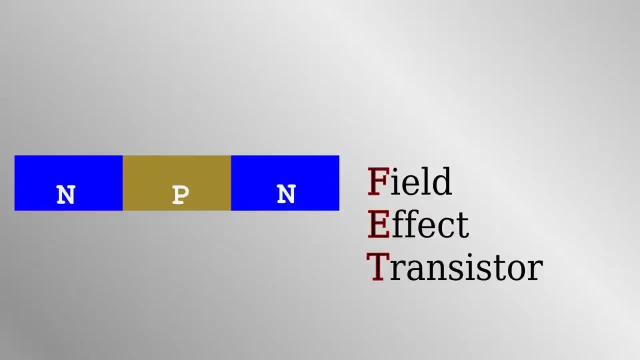 transistor. This can be thought of in simple terms as the electric field attracting electrons from the n-doped region, which has a surplus, to the p-doped region, which has a deficit. Near the semiconductor stack, we have a conducting electrical terminal. when it's at high voltage. 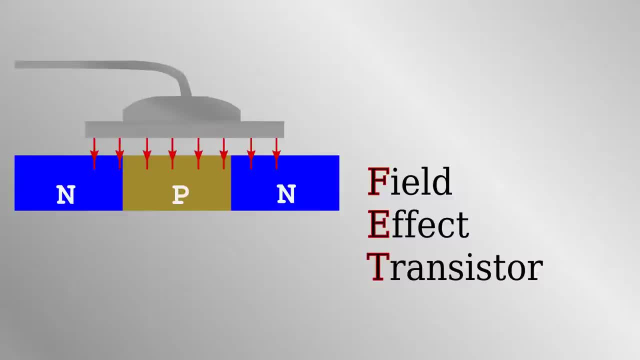 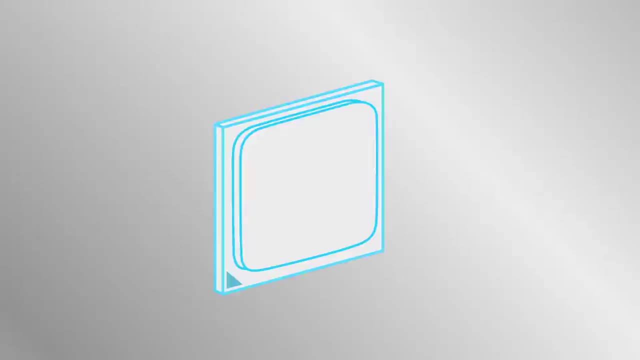 an electric field forms and the transistor conducts. But to stop a short circuit we need to add an insulating layer between them. The contact is metal, the insulator is silicon-oxide and finally we have the doped semiconductor, hence the term MOSFET. 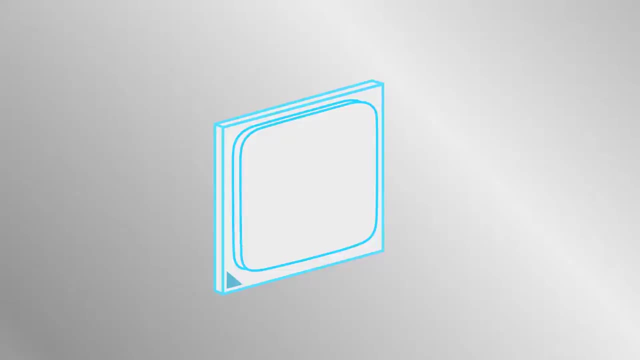 For a computer we need millions of interconnected CMOS pairs, and they must be small and close together so that electrical signals can travel between them quickly. Making a processor typically begins with a solid block of p-doped silicon called a die. Transistors are then created. 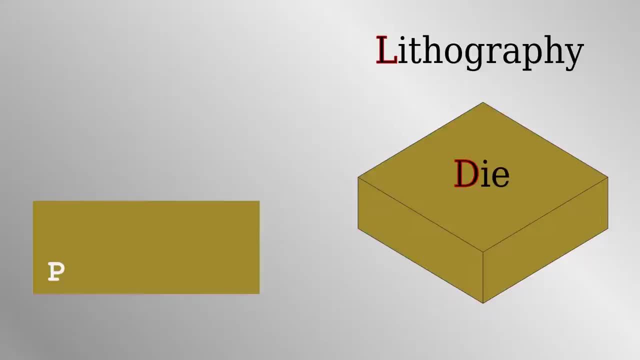 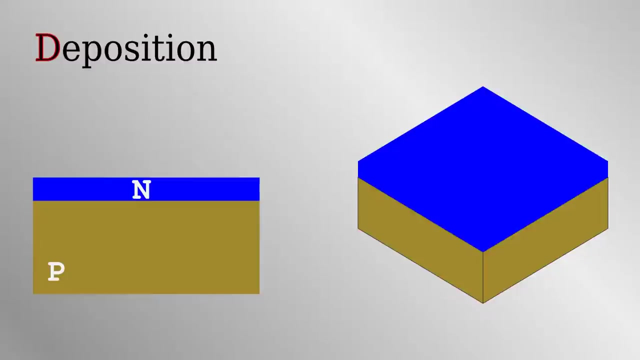 on top of the die by a process called lithography- writing on stone. There are two main techniques used in lithography. The first is deposition: chemically building up a layer of controlled, predetermined thickness across the entire die. This means that, for example, n-doped 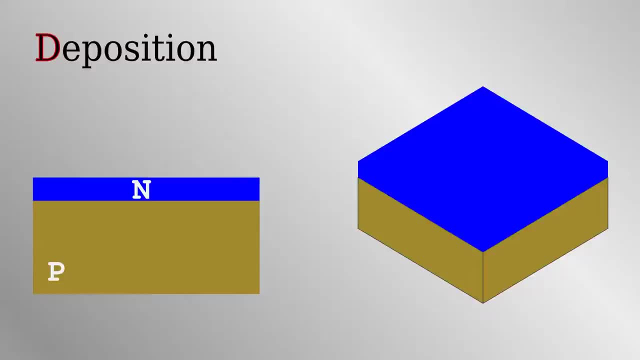 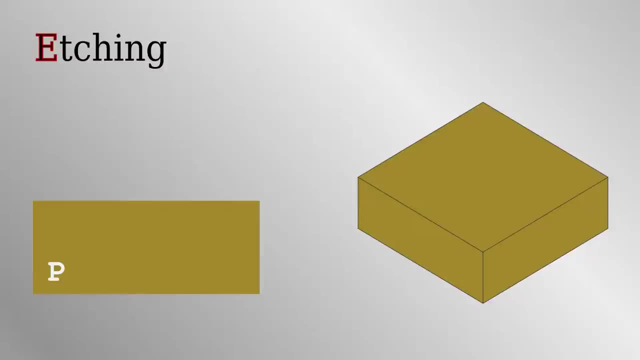 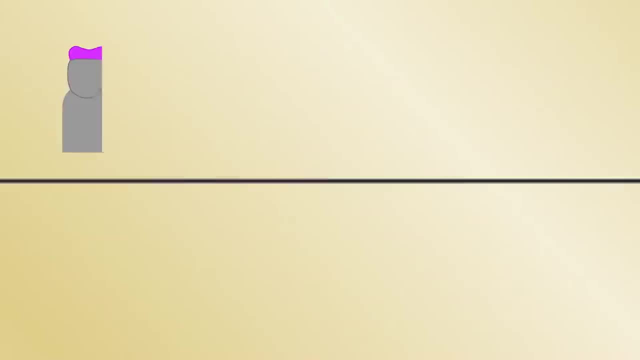 done by applying chemicals or hot plasma to the die. This is done by applying chemicals or hot plasma to the die. This is done by applying chemicals or hot plasma to the die. This is choosing a restaurant. Alice is happy when the restaurant serves burgers. Bob is happy. 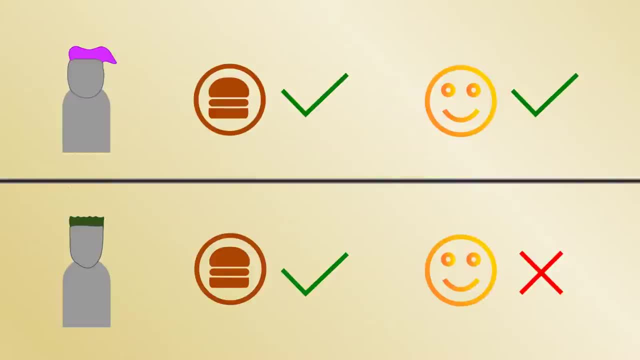 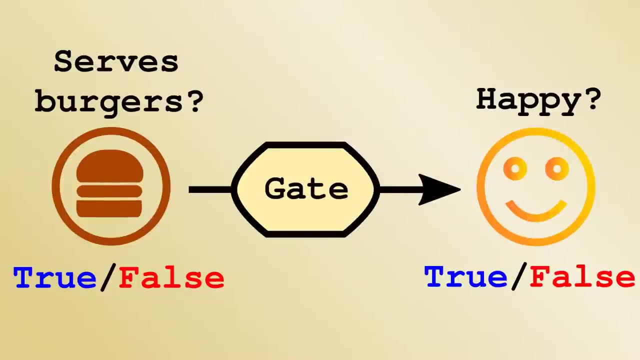 when the restaurant does not serve burgers. We can think of evaluating restaurants in this case as something called a gate, an object which takes a binary input- true or false, one or zero- and returns a binary output. In this case, the input is whether the restaurant has burgers and the output is if someone 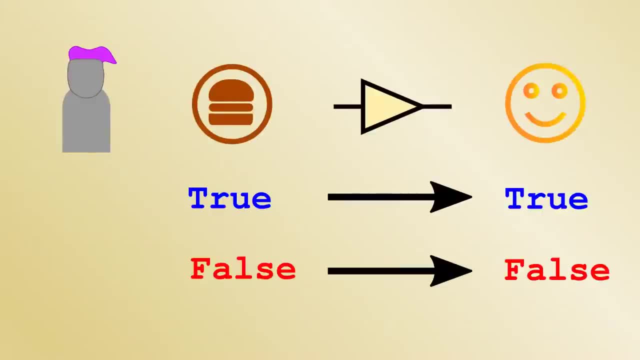 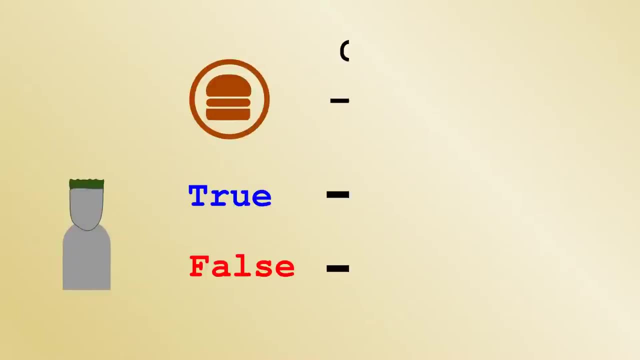 is happy with the restaurant. For Alice, the gate is simple. The output is the same as the input. In electronic terms, the circuit is just a connection. For Bob, the gate is what's unimaginatively called a not-gate. This is the symbol typically. 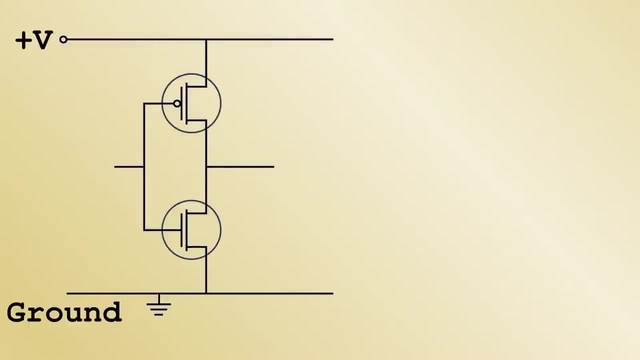 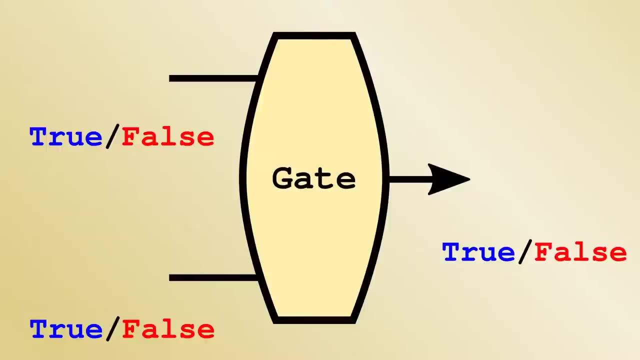 used to denote it In the previous section. we have seen how this CMOS pair acts as a not-gate. Let's consider a more interesting example. when the logic gates can have multiple inputs, Such gates have pretty straightforward names, as we'll see. 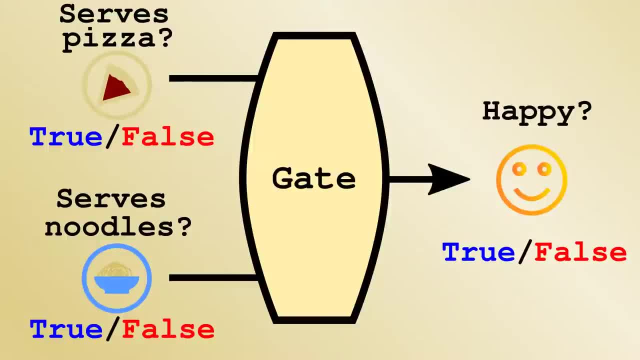 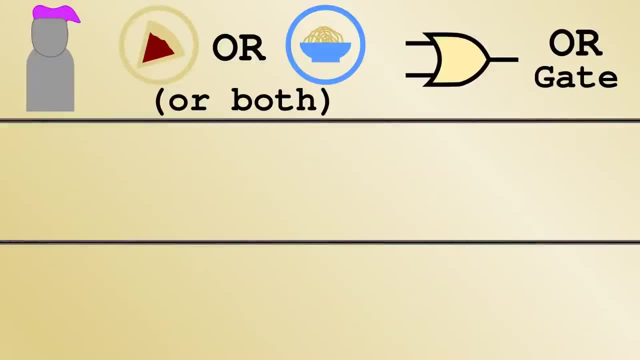 Now the friends are choosing restaurants which might serve pizza, noodles, both or neither. Alice is happy when the restaurant serves at least one of the two options or both. This idea is represented by what is called an OR gate. This is the symbol. 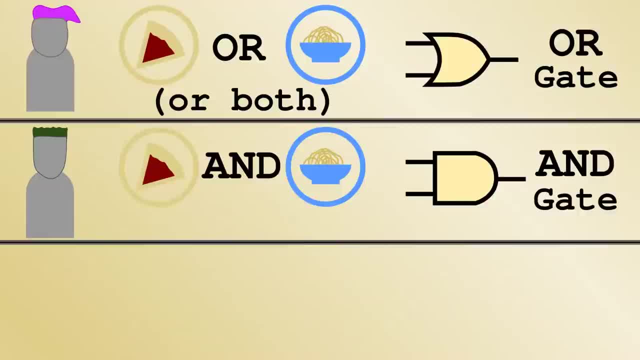 Bob wants choice, so he wants both pizza AND noodles on the menu, hence the AND gate. Charlie likes it if the restaurant serves pizza or noodles but not both. Let's say she thinks that they wouldn't do a good job if they weren't specialised enough. 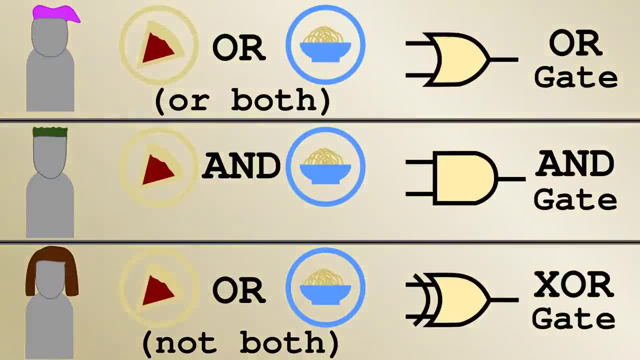 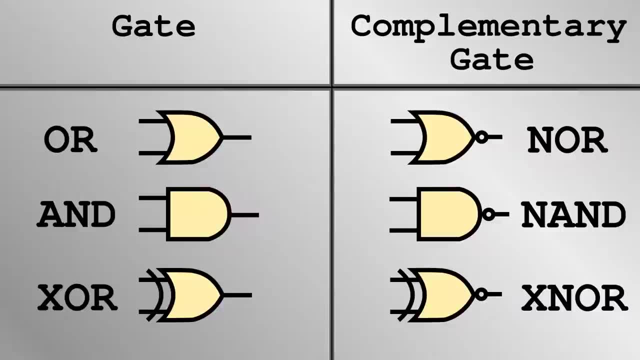 The corresponding gate is called exclusive OR XOR. Each of these gates also has a complementary gate, basically the same gate with a not-gate after it. For example, the NAND gate gives a 0 when all its inputs are 1, and gives a 1 otherwise. 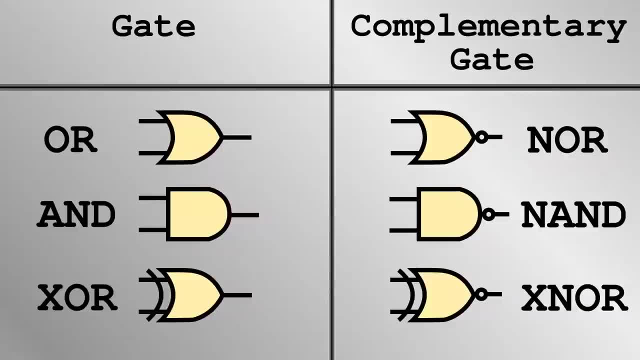 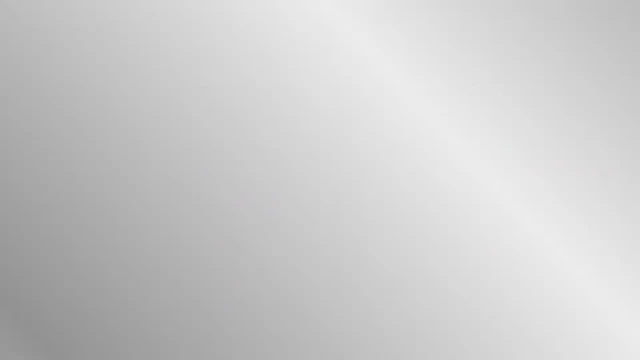 These complementary gates are denoted by the usual symbol with a circle at the output For a computer. these and all other possible gates must be implemented through CMOS pairs. Connecting two pairs as follows creates a NAND gate: The N-channel and P-channel transmissions. 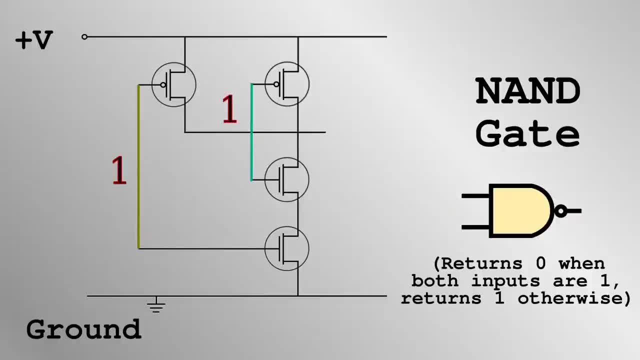 The N-channel transmissions and P-channel transistors still work in pairs. Only when a high voltage, or 1, is applied to both pairs of inputs do the paths to high voltage close and the path to ground opens, so a 0 is output. 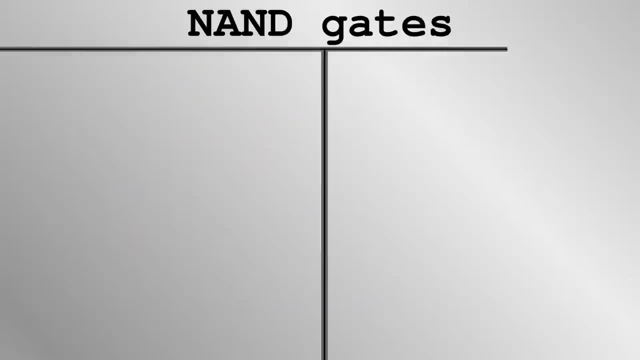 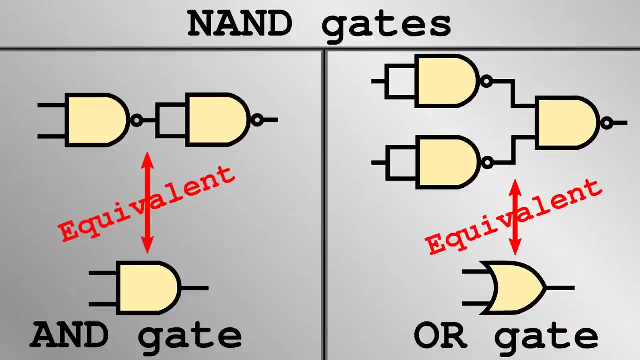 This is exactly the behaviour of a NAND gate. The NAND gate is important because it's what's called universal. This means that any other gate can be created out of NAND gates, as long as there are enough of them. Now there are more efficient ways to make certain gates, but in essence this means that 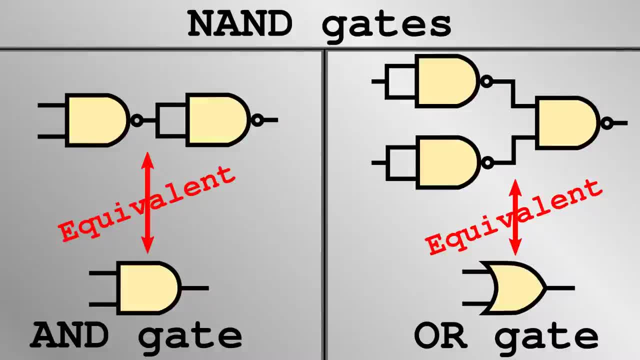 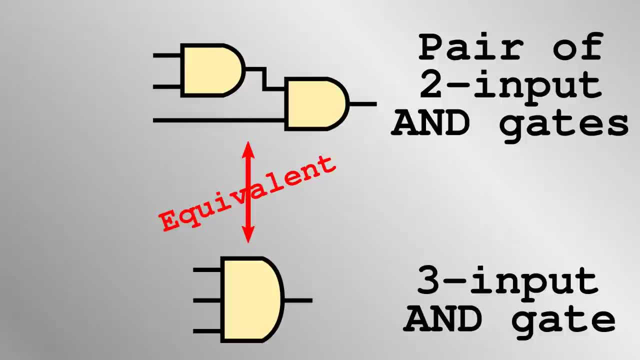 the problem of implementing logic gates is that the NAND gate can't be created out of NAND gates, as long as there are enough of them. There are also gates with three, four or as many inputs as necessary. For example, take two AND gates connected, as shown here, and they simply become a three. 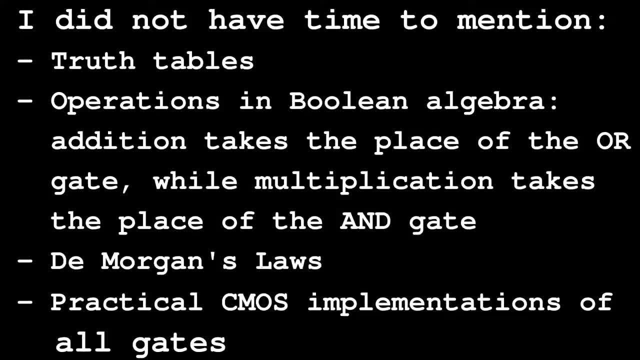 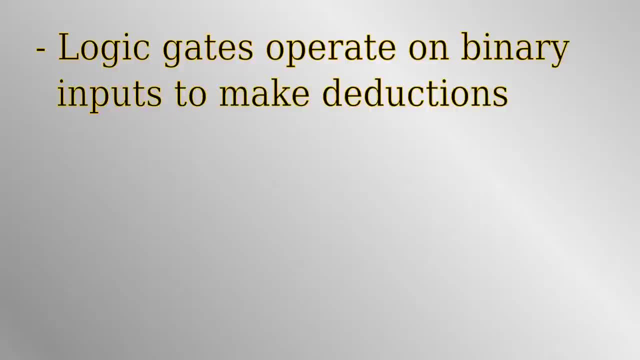 input AND gate, and so on and so forth. To summarise logic, gates are conceptual mathematical objects which allow us to make deductions based on binary true or false statements. For example, if it's true that today is Saturday or today is Sunday, then it's also true that 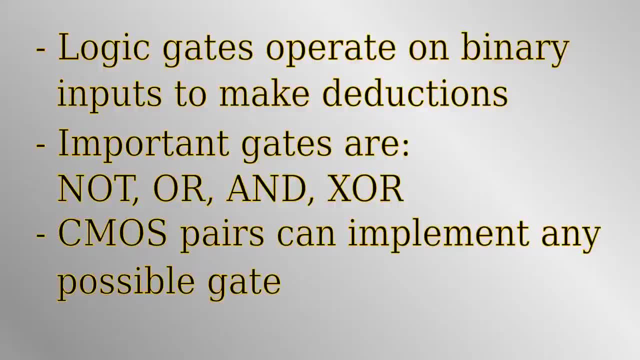 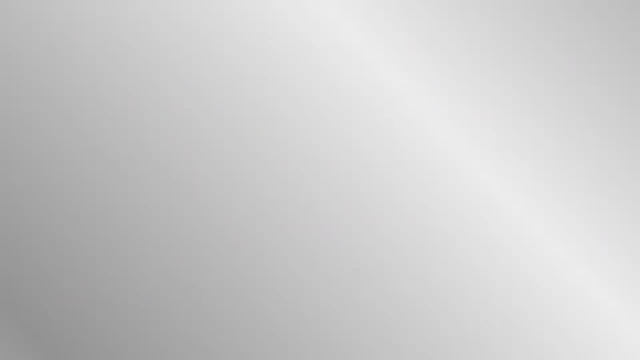 today is the weekend. We have seen how the CMOS pairs from the last section can be used to practically implement these gates in terms of electronic binary logic. Now we shall see how computers handled numbers and use logic gate networks to do arithmetic. We are all used to base 10 numbers, meaning that there are 10 digits, from 0 to 9.. 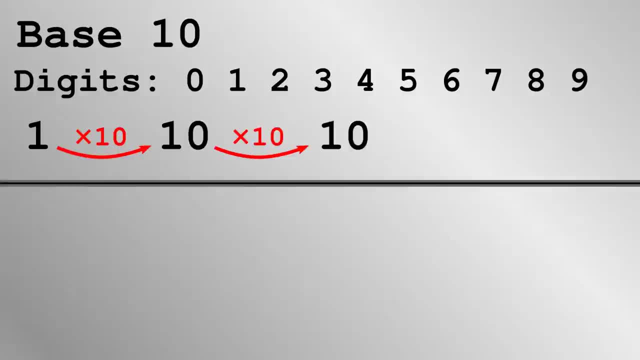 The digits represent multiples of powers of 10.. 10,, which are 1, 10,, 100,, 1000, and so on. Modern computers use base 2 numbers with just two digits: 0 and 1.. Binary digits are: 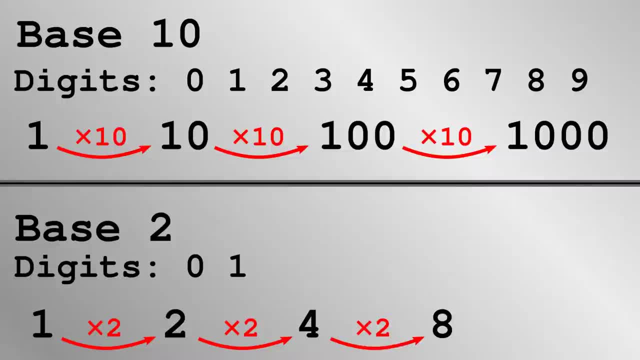 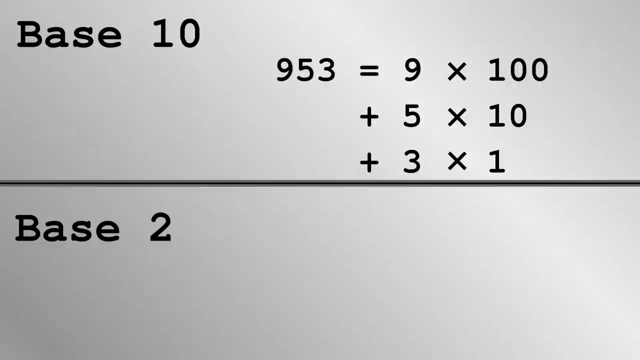 multiples of powers of 2,, which are 1,, 2,, 4,, 8, and so on. For example, in base 10,, the number 953 is 9 times 100 plus 5 times 10 plus 3 times 1.. 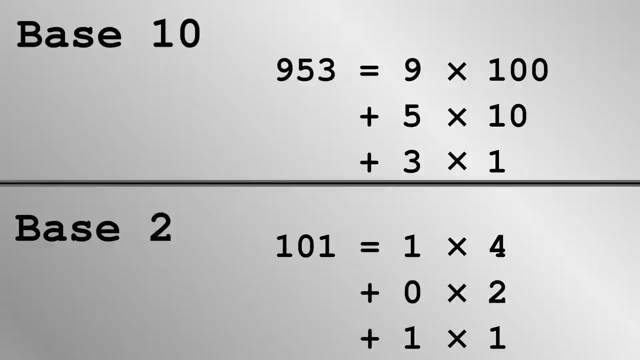 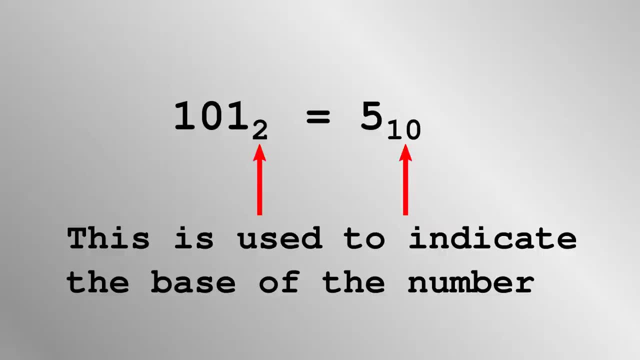 In binary, the number 101 is 1 times 4 plus 0 times 2 plus 1 times 1, which is 5 in base 10.. Any number in base 10 can be represented by a number in base 2, and vice versa. 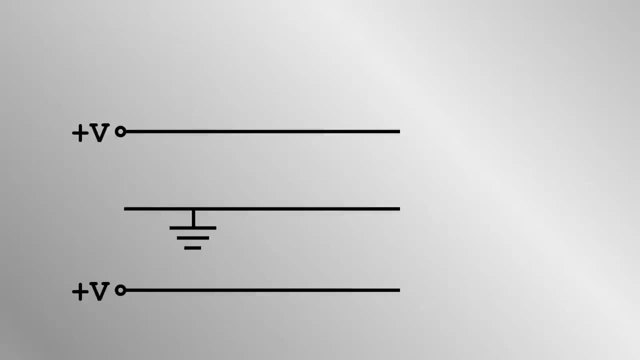 To represent the number 101,. three electrical tracks in order would have their voltage on off on. Each of these tracks carries a binary digit or bit. With three electrical tracks, this is called a 3-bit number. There are similarly 4-bit. 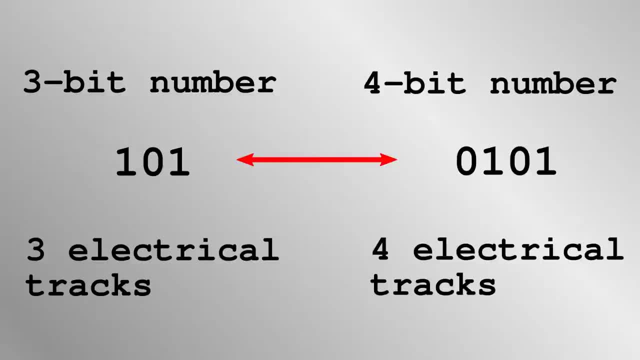 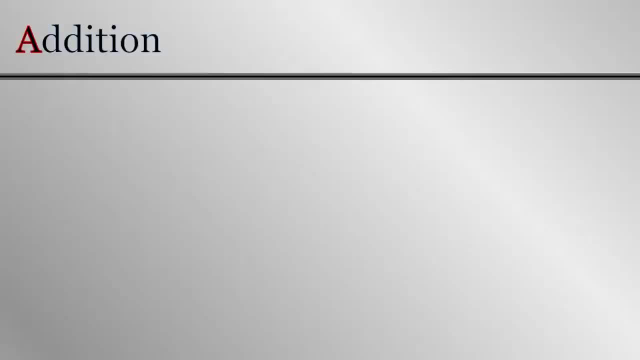 numbers, 8-bit numbers and so on. Of course, the 4-bit number 0, 1, 0, 1 is equivalent to the 3-bit number 1, 0, 1.. Let's consider adding together a pair of 1-bit numbers, A and B, to get C. 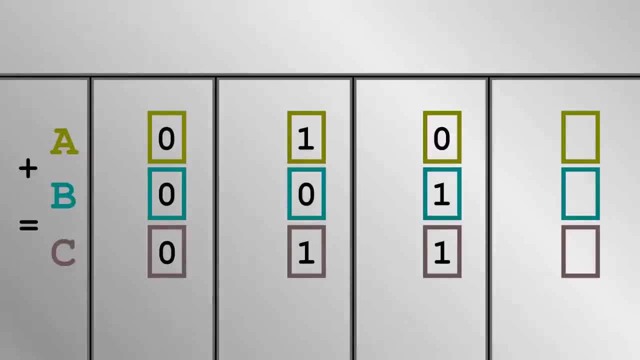 0 plus 0 is 0.. 0 plus 1 is 1.. What happens when we try to add 1 plus 1 in binary? The same thing happens when we add 5 plus 5 in regular base 10.. There is no digit big. 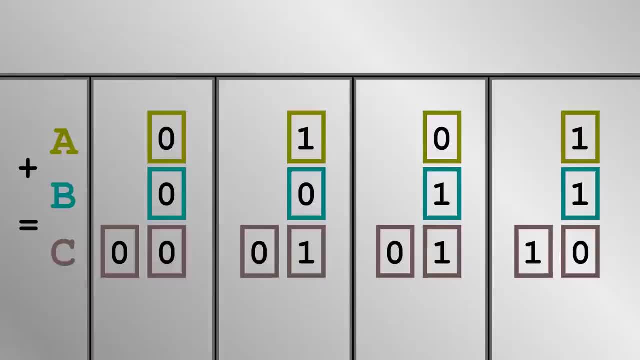 enough. so we put a 0 in that column and carry the 1 in binary. So to guarantee being able to store the result for any possible values of A and B, the result C must be a 2-bit number. The bit on the right is 1 when A or B is 1, but not both. This 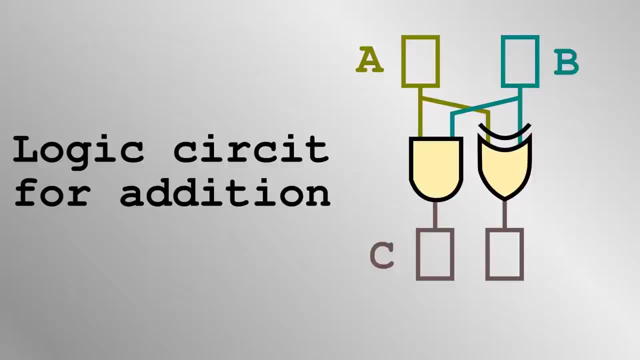 is the behaviour of the XOR gate. if you recall Charlie from the last section, The bit on the left is 1 only if A and B are 1, ergo the AND gate. Therefore, C is obtained by connecting A and B to gates like this. 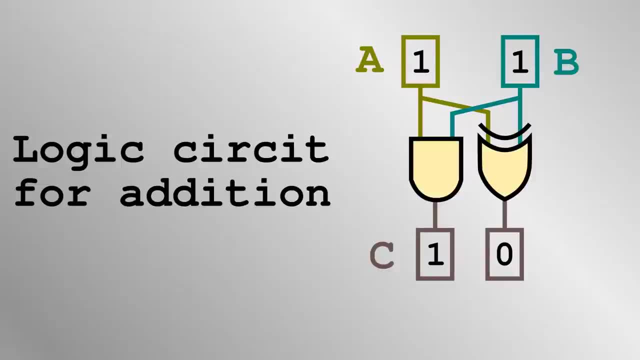 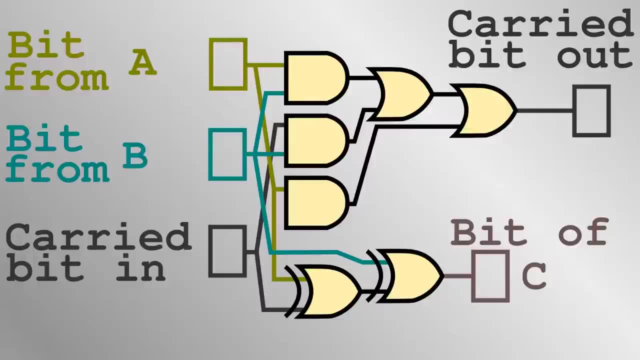 When adding numbers A and B larger than 1-bit. things get more complicated with 3-input gates because there is now a bit from A, a bit from B and a carried bit. As I said in the previous section, NAND gates are universal, meaning that any required gate network can be implemented. 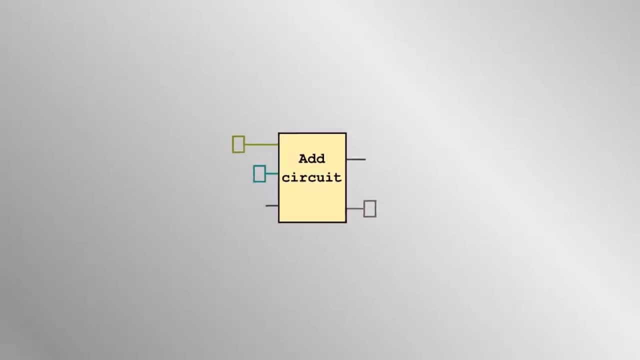 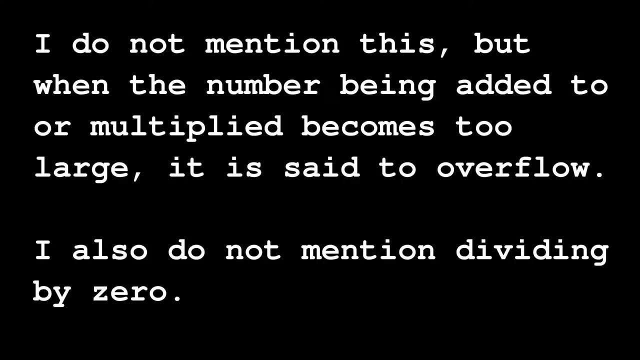 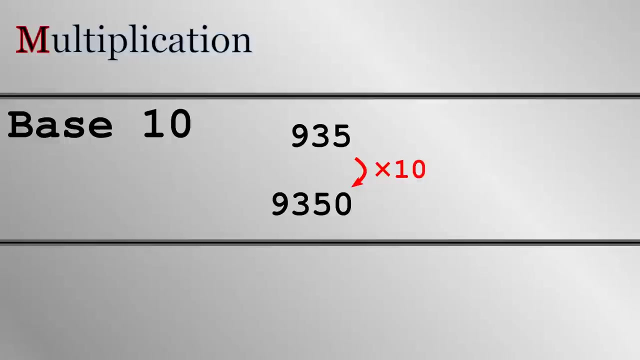 using enough of them In base 10, multiplying by 10 is easy: just add a 0 onto the end of your number In base 2, the same is true for multiplying by 1: 0 in binary or 2 in base 10.. So multiplying. 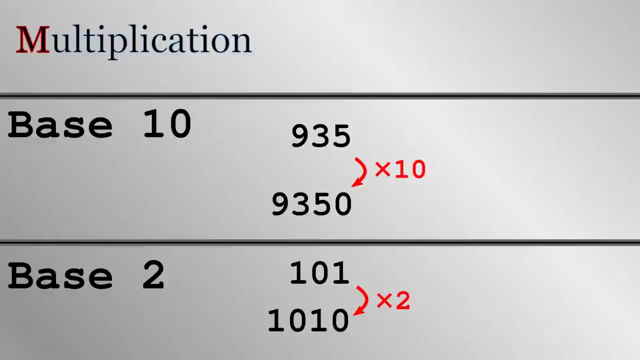 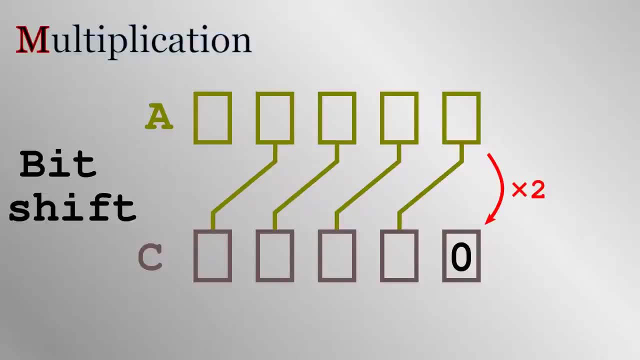 by the numbers 1 0, 1 0 0, 1 0 0 0 in binary just involves shifting each bit to the left and putting a 0 on the end, which is unimaginatively called a bit shift. 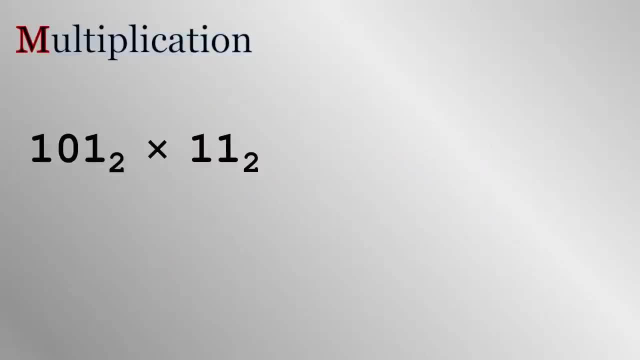 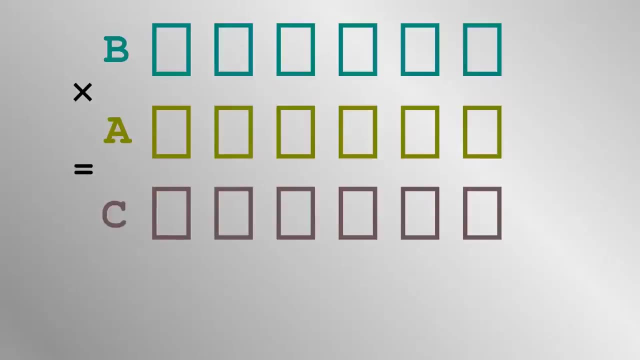 What about multiplying by an arbitrary number, Say for example, 1: 1? in binary This is the same as multiplying by 1, 0,, multiplying by 1, and adding the two together. So binary multiplication of A by an arbitrary number B works as follows: 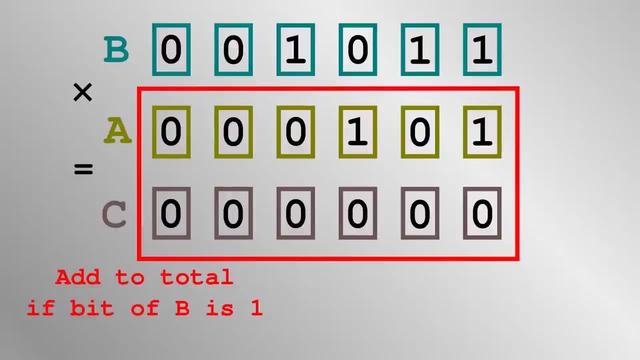 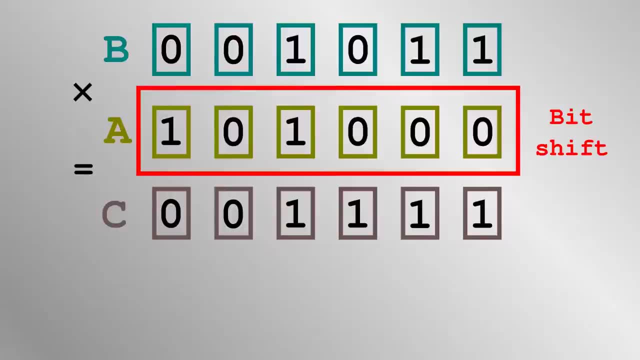 Begin with 0.. If the rightmost bit of B is 1, add A Bit. shift A once, and if the next bit of B is 1, add this to the total. Continue for every bit of B. Computers also rely on making comparisons of numbers, such as: 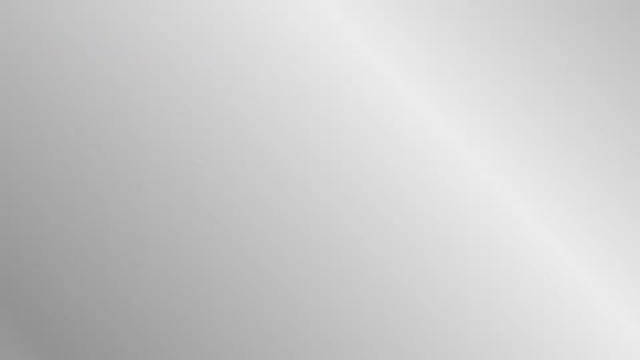 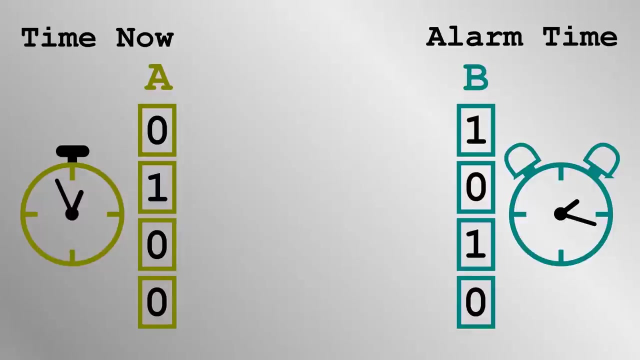 Is A equal to 1? Is A equal to B, Is A greater than B, And so on. The computer might have the current time in seconds stored as a binary number, A updated every second, and the time to set off an alarm stored as B. The alarm would be made to go. 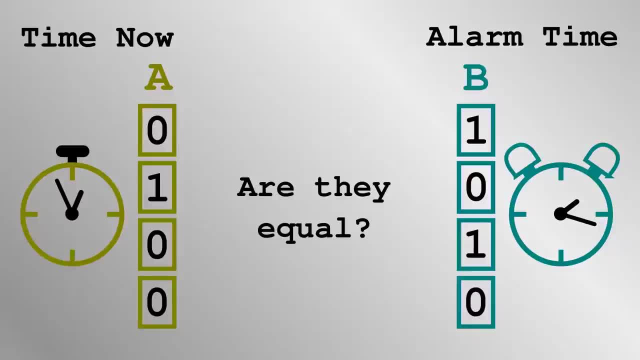 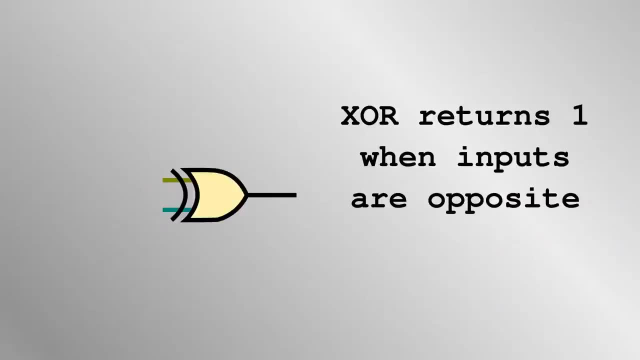 off when A is equal to B. To do this, the computer must check that every bit of the number A is the same as the corresponding bit of B. So the XOR gate returns 1 when an input is 1 and the other input is 0, in other words: 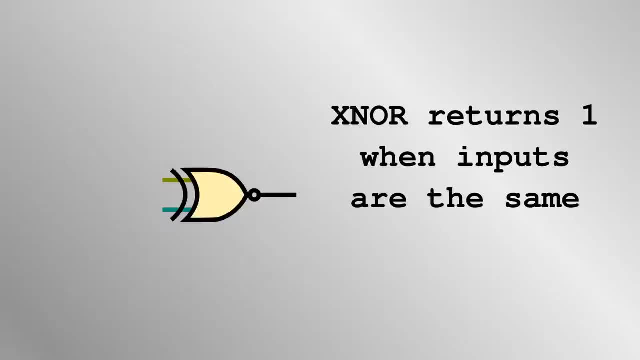 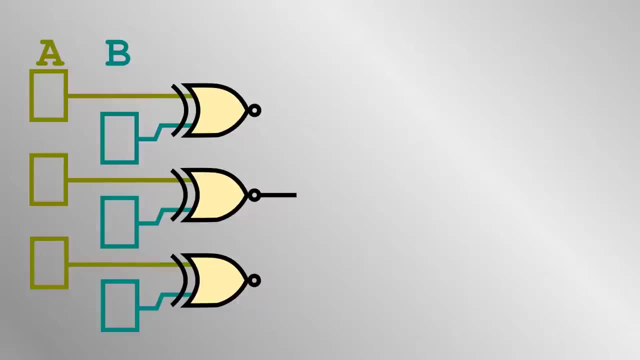 when its inputs are different. The XNOR gate, which is the complement to the XOR, means it returns the opposite to the XOR, therefore returns a 1 when its inputs are the same. A bunch of XNOR gates applied to each pair of bits of A and B return whether those bits 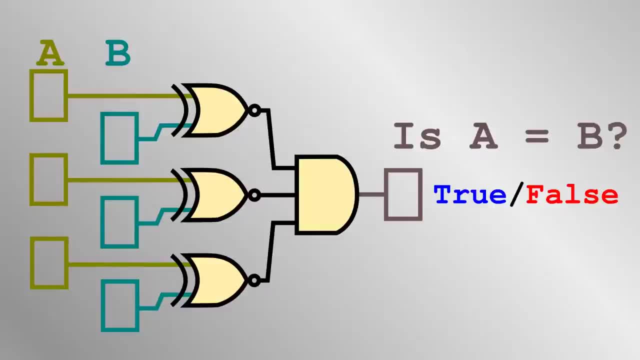 are equal or not. The AND gate returns a 1 when all its inputs are 1.. So applying it to the XNOR gate returns a single bit, which is 1, if, and only if, A is equal to B. There are also ways to implement subtraction, division and other comparisons, all using 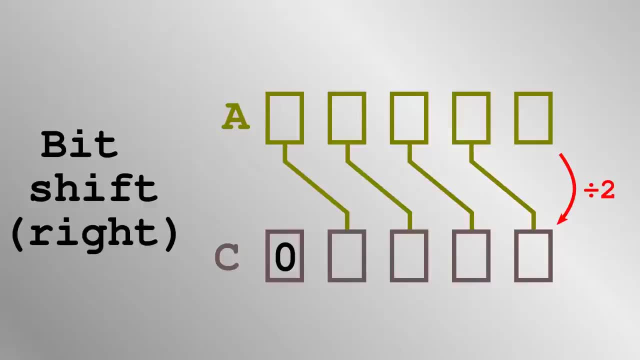 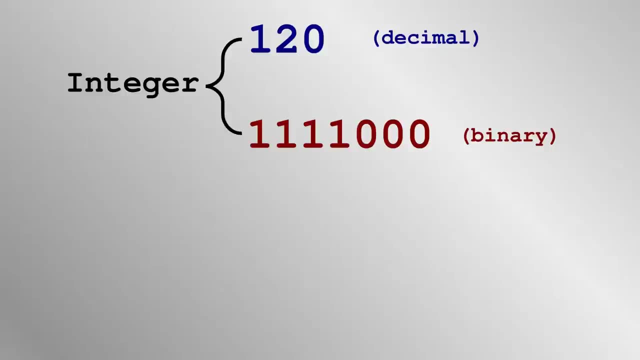 gate networks, For example, bit shifting the other way divides numbers. These are all implemented using transistors edged on a chip. Just a note: when I say the word number in this video, I am referring to an integer or whole number. 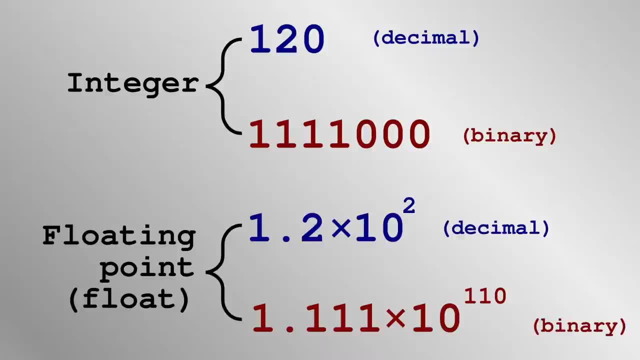 There is also a way to store fractions in a binary version of scientific notation called floating point numbers or floats. I won't go into how they work, but the general principle outlined here still applies. To summarise, a sequence of binary on-off electrical signals is used by computers to 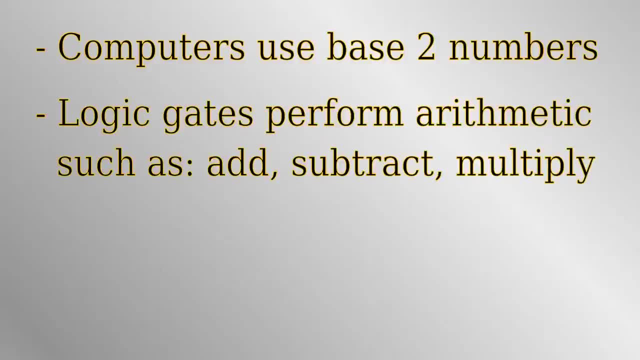 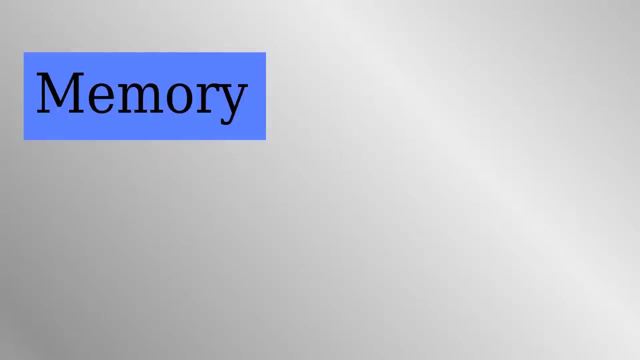 represent a number in base 2. As opposed to base 10, which is used by people day to day. Networks of logic gates can be used to add, subtract and compare binary numbers and, with a few extra steps, multiply and divide them too. 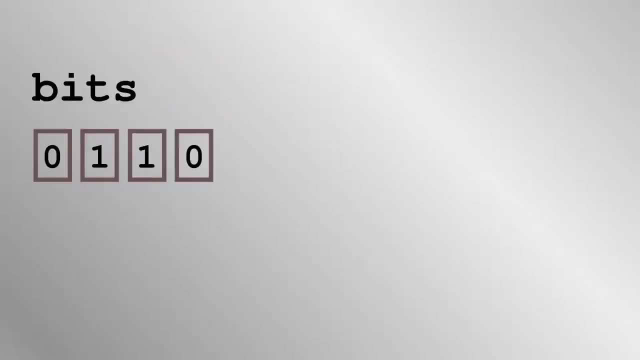 We have seen how circuits composed of transistors can be used to implement addition and other algebra for any number with arbitrary binary digits or bits. If you want to build a computer, we would have to choose exactly how many electrical tracks and gates to have available for representation. 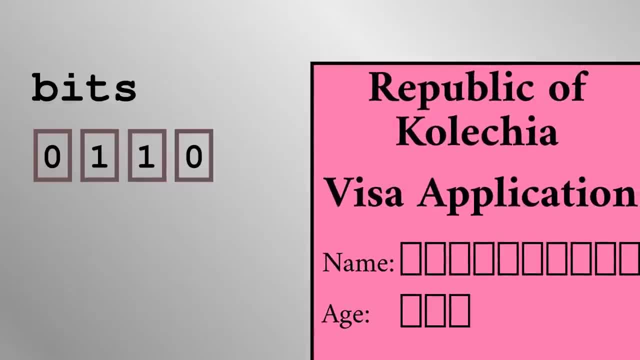 So if you want to build a computer, we would have to choose exactly how many electrical tracks and gates to have available for representation. This is like when you're filling in a form and it has a set number of boxes physically printed on it for putting in your age. 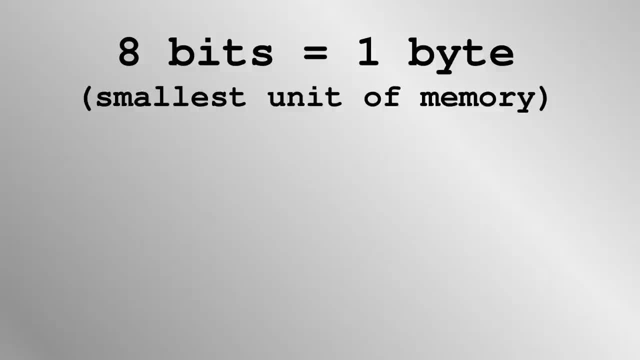 For commercial computers this is always a multiple of 8.. 8 bits are called a byte. The computer will have adder circuits and so on of the types I described in the last section, which take 1 byte or 8 bit, numbers 2 byte or 16 bit, numbers, 4 byte or 32 bit. 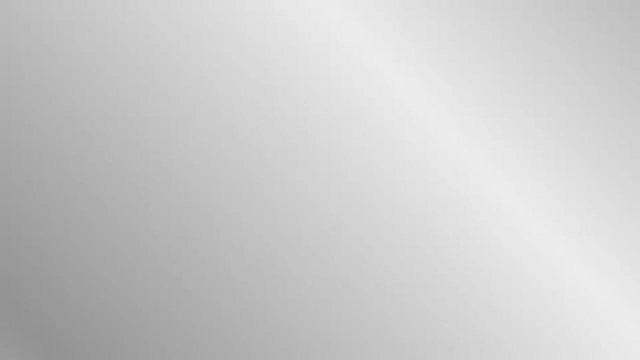 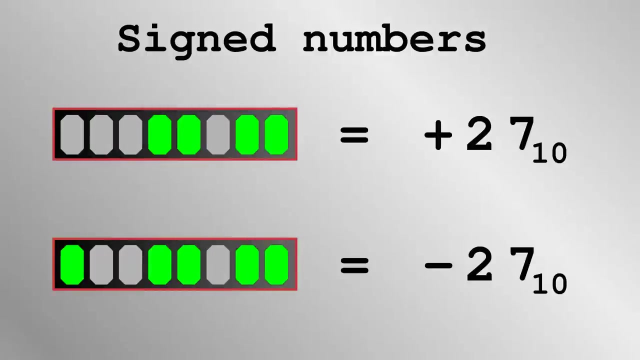 numbers as inputs. No matter how many bytes a number is comprised, one of its bits can be set aside to denote a plus or minus sign. When a number is signed in this way, if the leading bit is 0,, then the number is positive. If the leading bit is 1,, then the number is negative. 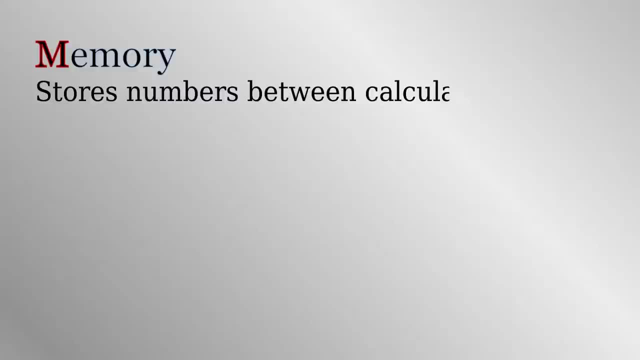 As anyone who has ever taken a mathematics exam knows, it's important to store your workings. Whichever operation a computer undertakes, the inputs and outputs must be somehow stored. To do this, a type of circuit called a latch is used. Once it has latched, it will stay that way for a long time and can therefore be used. 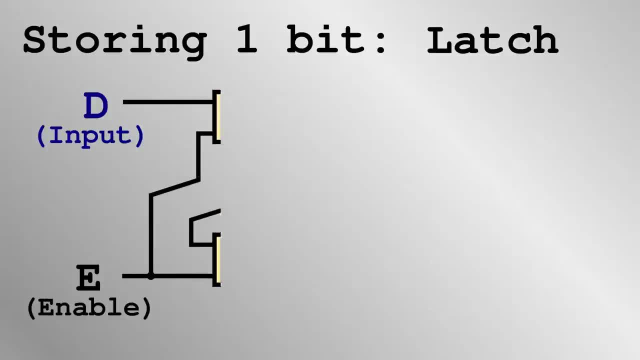 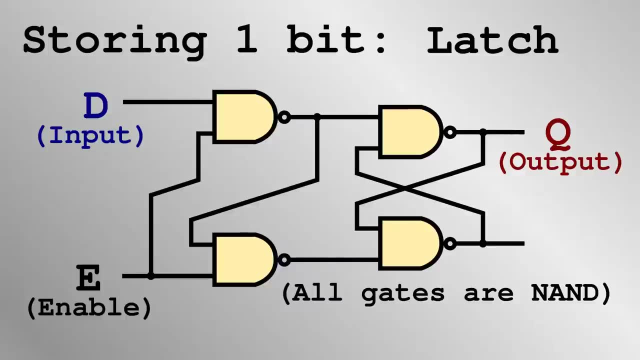 to store a bit of data, 8 latches store a byte, and so on. This is an example of what's called a D latch comprised of NAND gates. You may notice that this looks rather strange. Before we have seen gates in a strictly sequential manner, where the output of one gate goes: 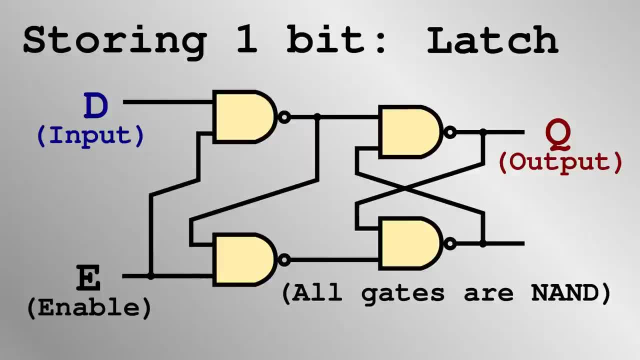 directly to another. Now there is an output from one going to the input of another, but then the output comes right back. It is this kind of interconnection that allows this network of gates to hold and retain its output value, 0 or 1.. 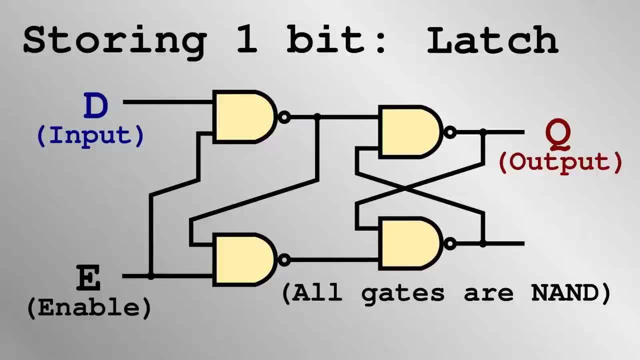 Nothing will change unless the E or ENABLE input is 1.. When ENABLE is 1, whatever bit is applied to D will propagate to the output. The computer will carry out an operation enable a bunch of latch circuits to store the output and then switch the ENABLE back off. 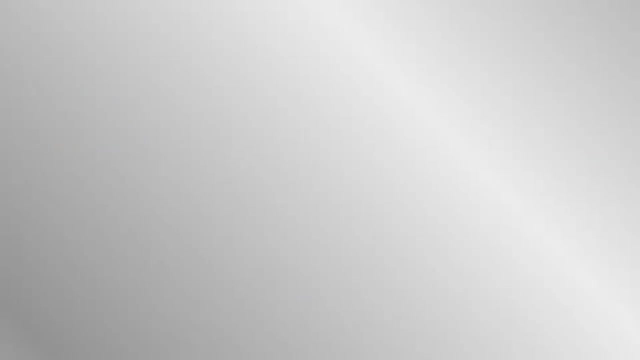 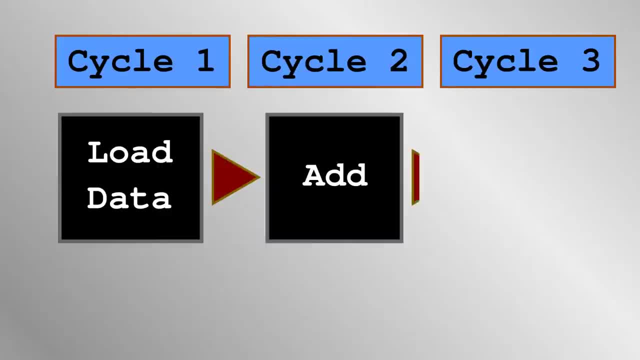 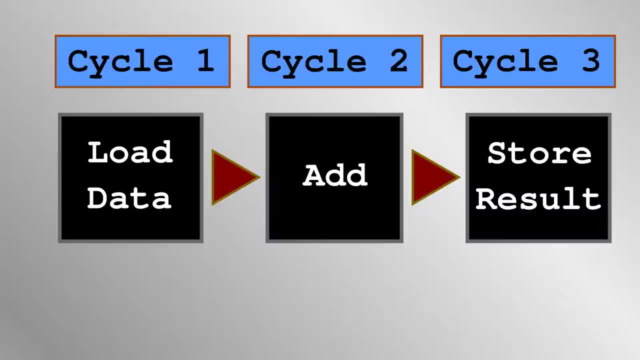 An ADD circuit of the type we looked at in the last video will store a byte of data as long as it's required. the next clock cycle. finally, on the third clock cycle, the output register gets an enable signal and stores the result. actually, most operations take much longer than one or even three clock. 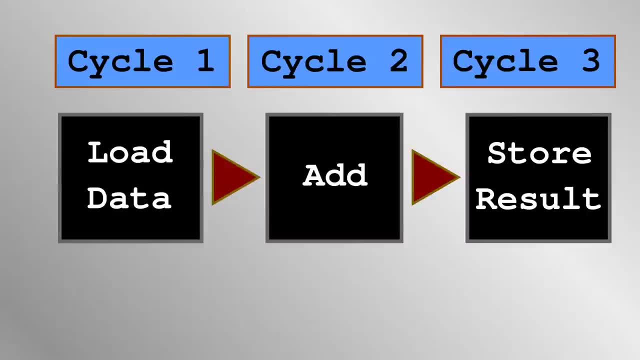 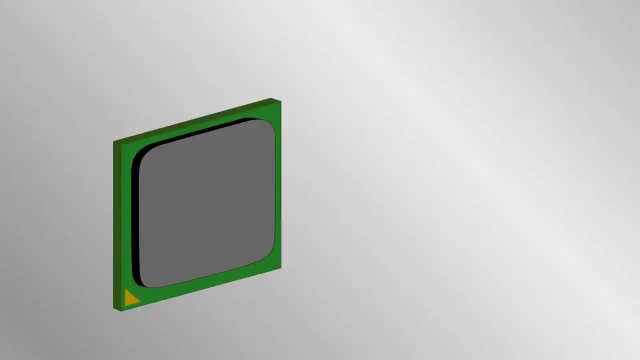 cycles to carry out. we have seen in the previous section that multiplication takes several adding steps to accomplish. nonetheless, whether it takes one or a hundred cycles, the clock is still used to synchronize when an operation begins until the output is ready, or the so-called arithmetic logic, that is, all the arrays of logic gates which do addition and subtraction, is physically located. 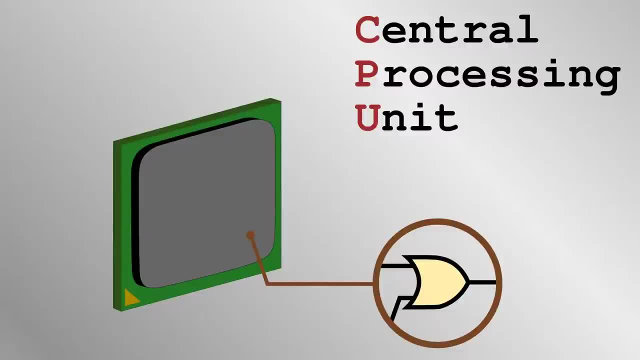 together with the registers on a chip called the processor or central processing unit. there are also circuits in there called the cache, which nowadays can store tens of kilobytes of data as the intermediate stages of calculations, for example. there is a need for a larger and longer 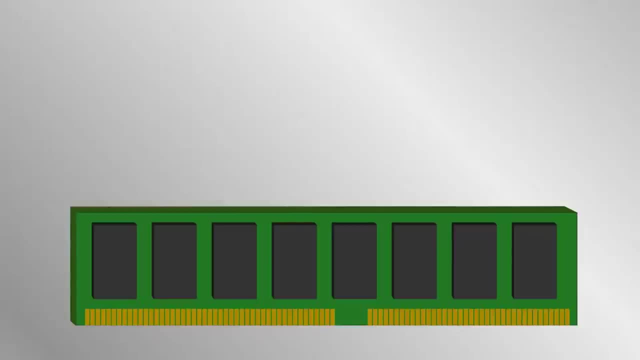 term way to store many more bytes of data than the registers and the cache. computers have separate physical chips of rand and gps chips, of the gps and gps chips, of the gps and gps chips, of the gpch. access memory or RAM, which makes use of capacitors to store this data. If a 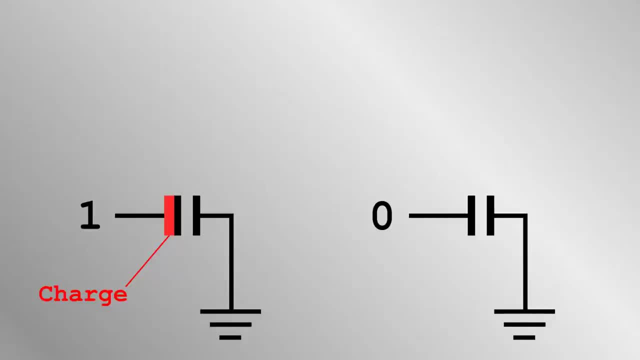 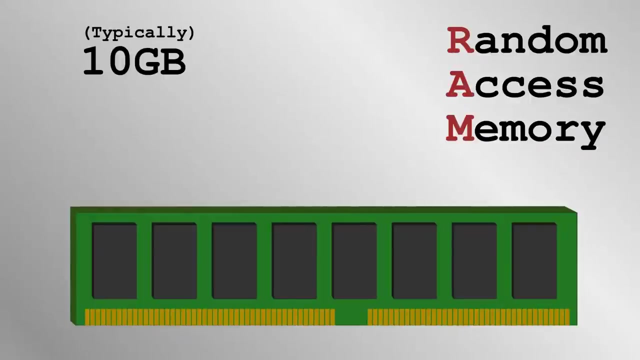 capacitor is charged, it has a high voltage and therefore a value of 1. If it's discharged it has zero volts relative to ground and so is zero. The charge leaks or is lost over time, but is topped up by the memory circuits as long as the computer is powered. A typical laptop computer has tens of gigabytes or 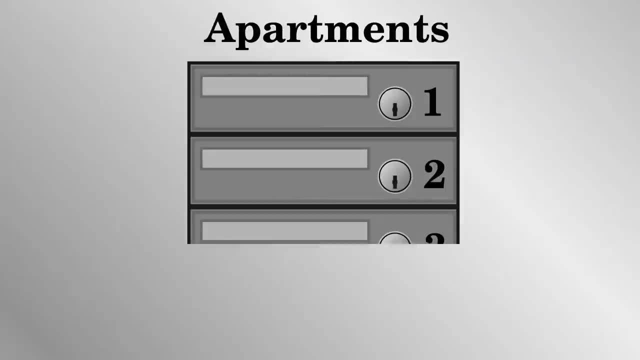 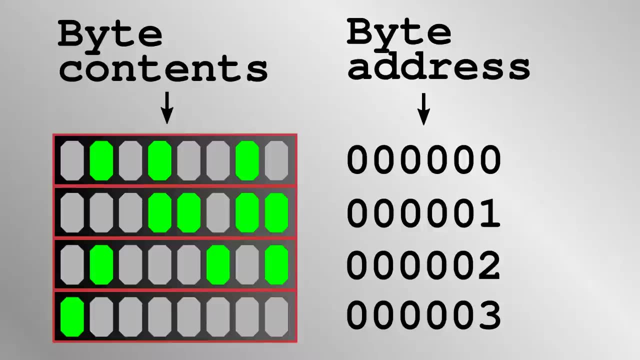 billions of bytes of RAM. Every byte stored in RAM has its own address, like a post box in an apartment block. The address is itself a binary number. The RAM has many transistors forming gate networks which ensure that when it receives the address in binary format from a processor, it then returns the. 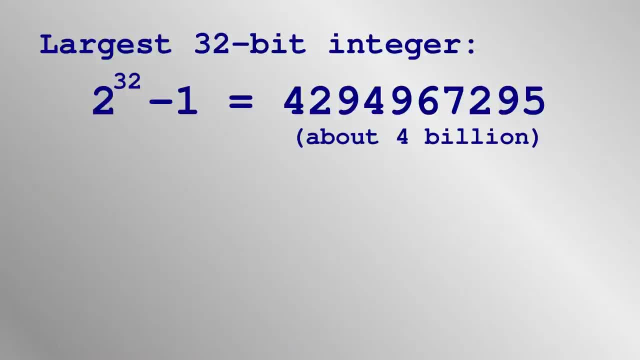 bytes stored at that address. Until recently, computers wouldn't usually have more than 4 gigabytes of RAM. Each of those bytes requires a unique address, so memory addresses were 32-bit numbers. Such 32-bit numbers go up to just over 4 billion, So that used to be the number of bytes stored in a processor. 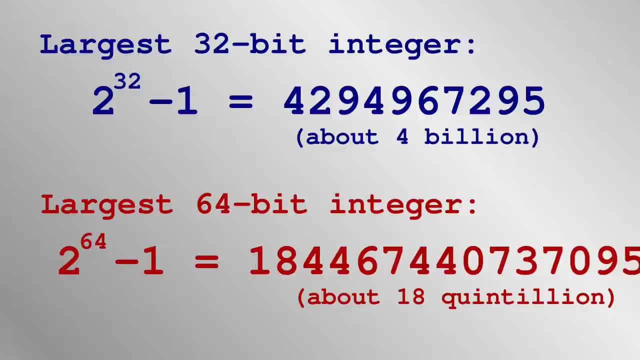 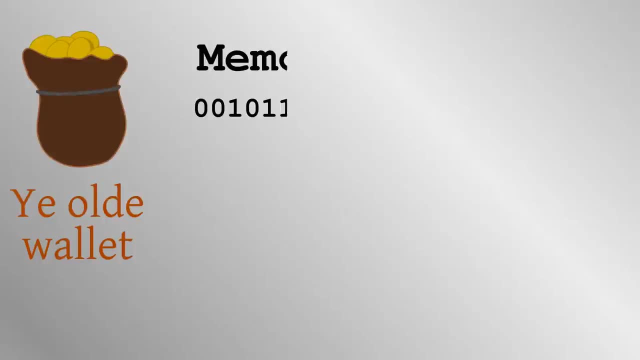 When RAM got bigger, there effectively weren't enough addresses, so now 64-bit numbers are used for memory addresses. This is the difference between 32 and 64-bit programs. So let's say you're playing a video game where you have a number of coins in your wallet. The video game will keep track of the. 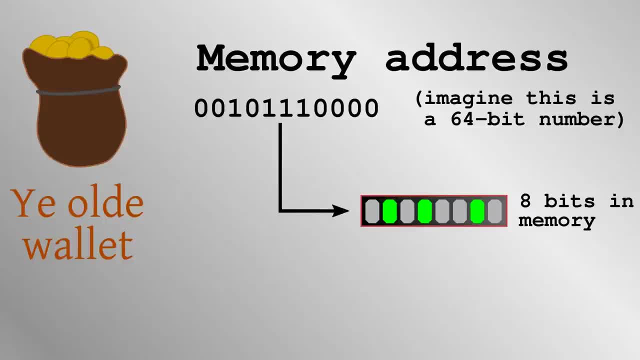 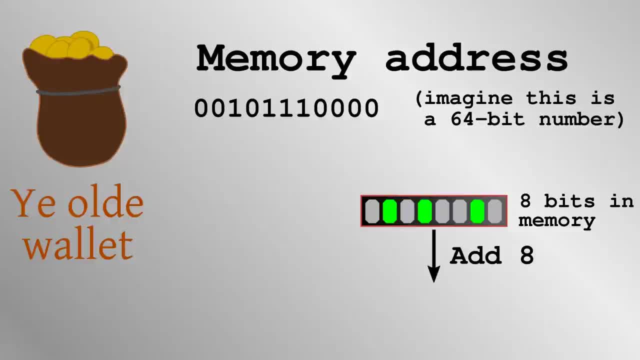 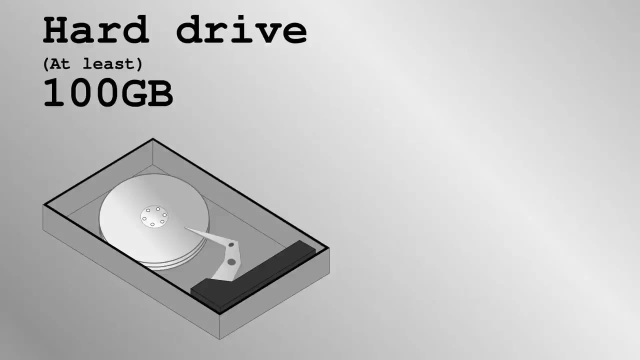 corresponding to 8 and base 10 into the other register, add them together and put the results back into the address with the wallet total. We will look at this in more detail in the next section. Computers also store huge volumes of data on hard disks for decades at a time. even without power, A hard disk is covered in. 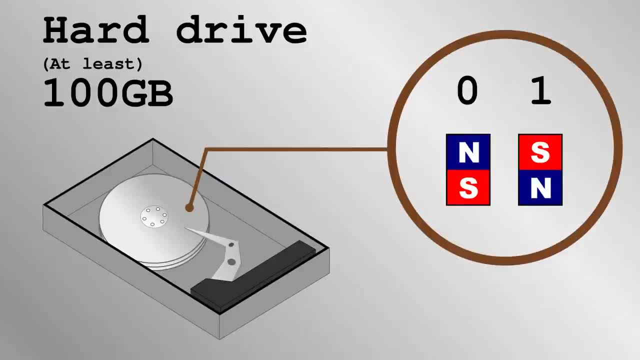 tiny magnetic domains which can point up or down corresponding to 1 or 0.. As the disk spins, a sensor head can either passively read off the orientation of the magnets or uncompressed by a gather. As the disk spins, a sensor head can either passively read off the orientation of the magnets or 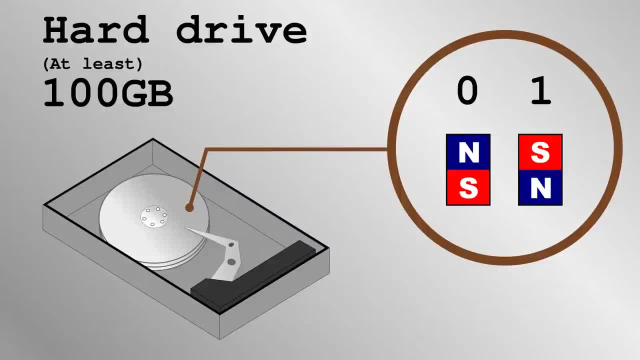 bits or actively flip the orientation of the magnetic domains to write data onto the disk. Each of the bytes also has its own separate address. A laptop or personal computer can store hundreds of gigabytes on a hard disk. There are other technologies like flash memory. 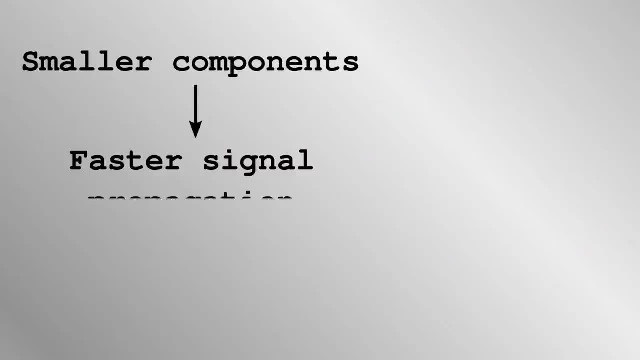 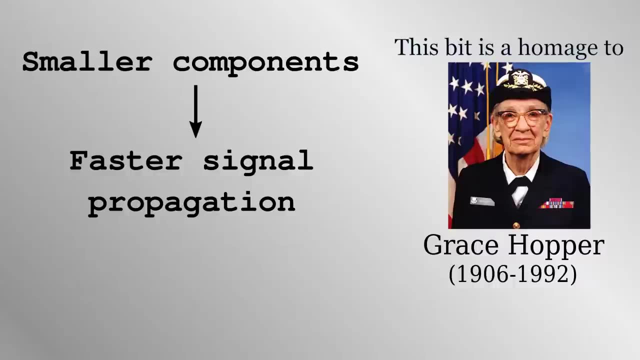 DVDs and so on that I won't go into here. The fundamental limit on how fast a computer can do operations is the speed of light, which can go about 15 centimeters or half a foot during a typical computer clock cycle. so it takes multiple cycles for a computer. 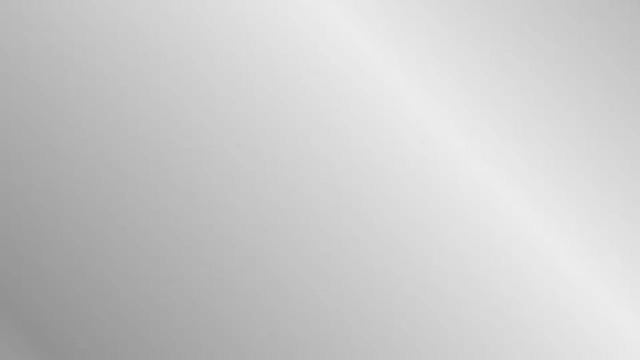 larger than that to fetch any data Realistically. transistors switch much slower than that, while a hard disk takes time to spin up and scan to read the data. In terms of types of computer memory, the cache is small but quick to access. 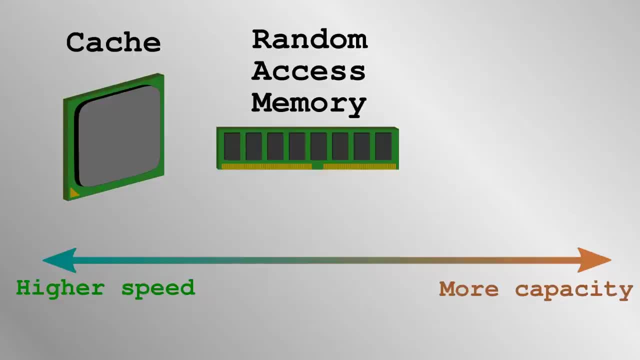 The RAM stores many more bytes of data, but takes longer to read. The hard disk takes the longest to read, but stores a lot of data almost permanently. So are there any things that are more important than a hard disk? a trade-off between how quickly the data can be retrieved and how much can be stored From now on? 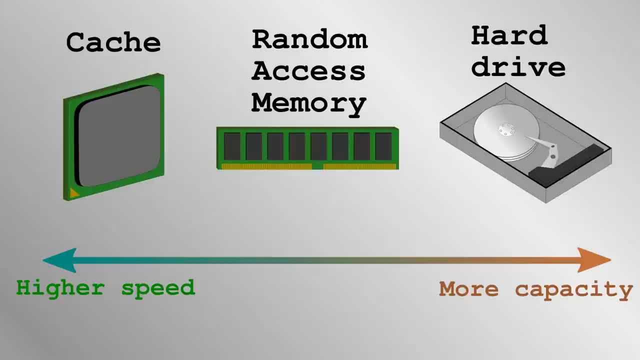 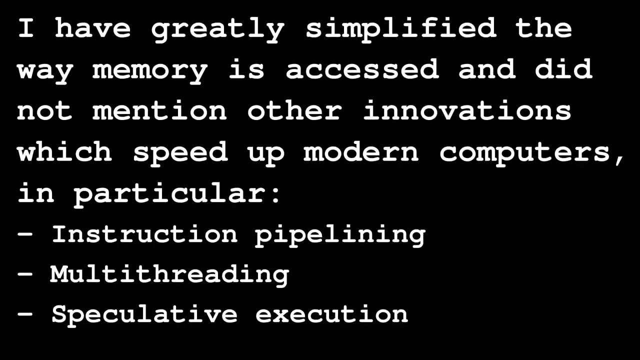 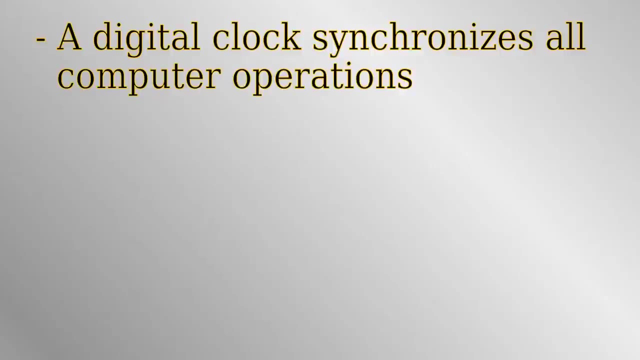 in this video I will explain things as if the computer just has a single pool of memory which it can instantly read. In reality, things are more complicated, as I've just described. To summarise, computers have a clock which synchronises the operations being performed. 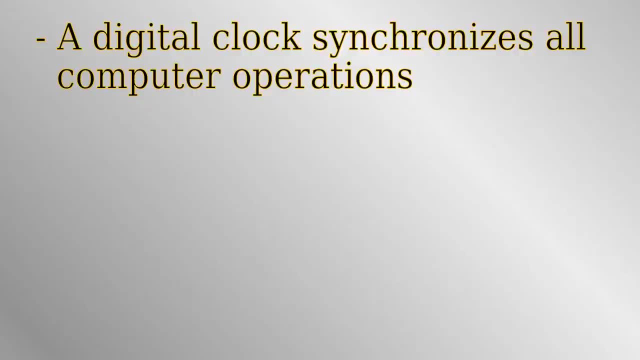 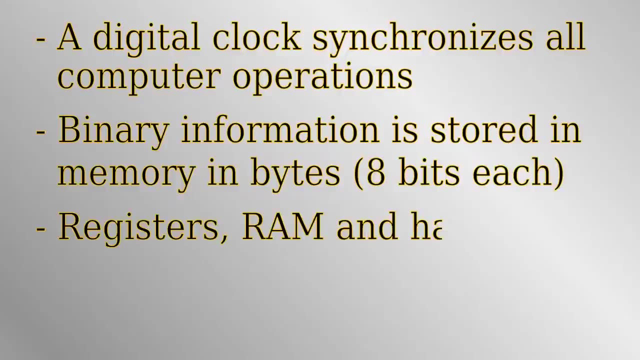 and ensures that there is enough time to finish performing one operation before starting another. Computers process. binary numbers in groups of eight bits, called a byte Registers, are used to store numbers during computations and at other times numbers are stored in the cache, in random access memory and on a hard disk. Each byte in memory has its own unique address. 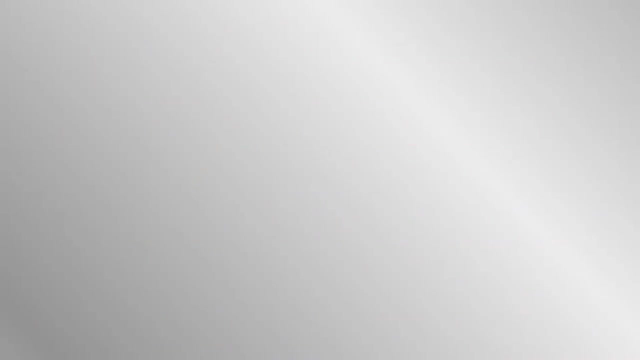 which is itself a binary number. We have a way of implementing binary operations and storing the results, but the computer will not be able to do so. The computer needs a way to determine which operation to use, and when This is called an instruction. There are instructions such as add two numbers and copy this number Computers use. 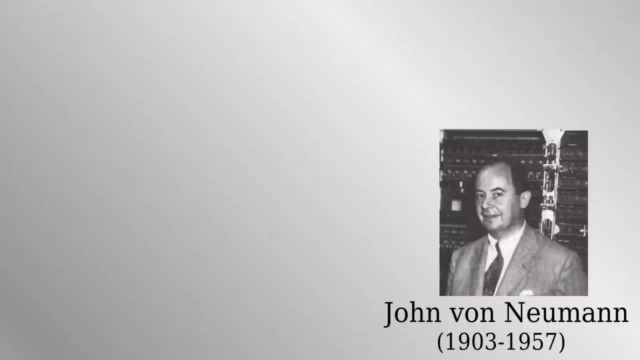 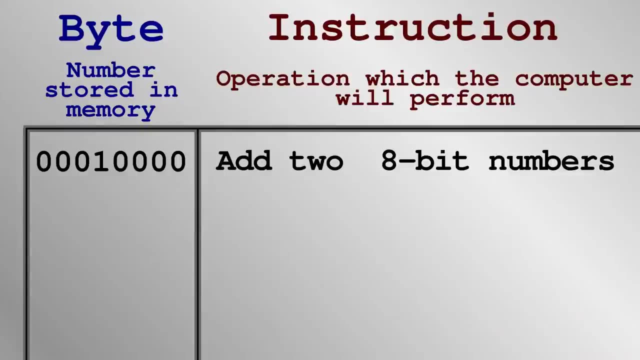 what's known as the von Neumann architecture, which means that the instructions are stored in memory as binary numbers amongst other data. For example, the instruction number 16 in base 10 or this byte in binary might mean add together two 8-bit numbers and store the result. Instruction number 17 might 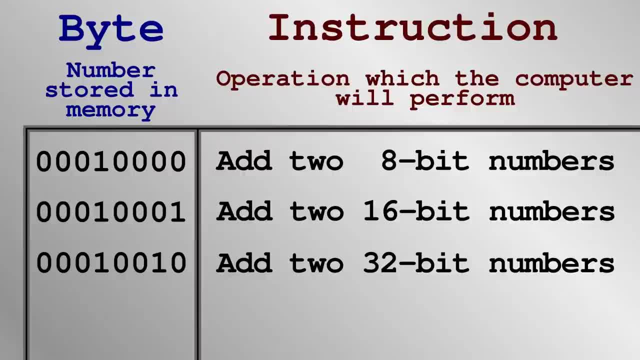 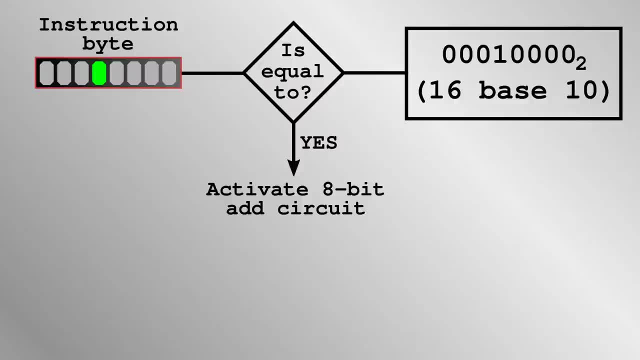 be the same but for 16-bit numbers and so on. When the computer encounters an instruction, it will use a comparison circuit, which we looked at in a previous section, to switch on the logic circuit for the necessary operation. If the byte is equal to 16, switch on the add circuit. How does the computer know when a 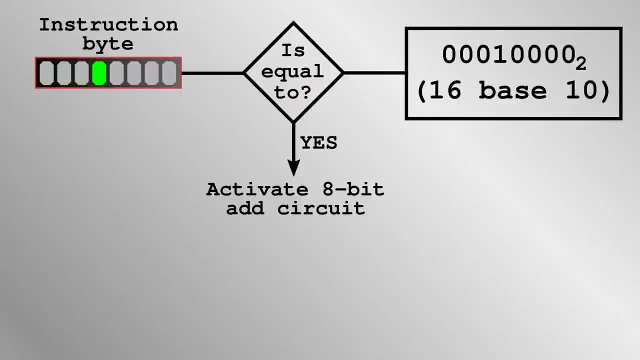 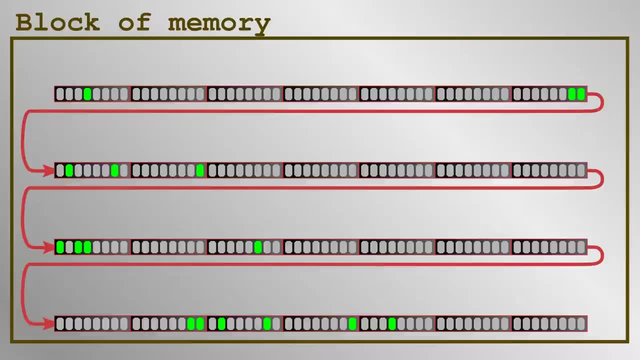 byte is an instruction or not. 16 might be the instruction to add, or it might be the number of coins in a video game. Well, everything has to do with the precise order in which the bytes appear in memory. First comes the instruction byte. If the instruction is to add, the computer will need. 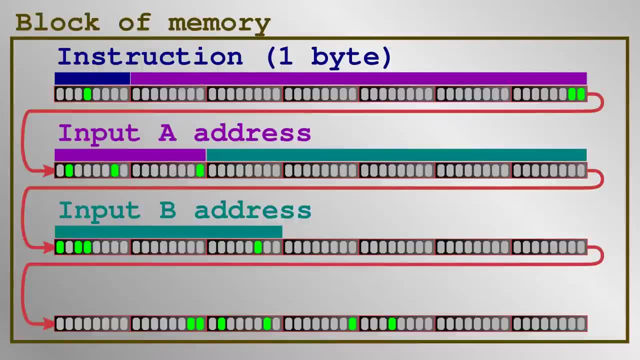 the two memory addresses of the things being added and the memory address where the result is to be stored. Remember that memory is like post boxes for a big apartment building with a unique address on each byte. In the case of modern 64-bit systems, addresses are eight bytes long. therefore, the 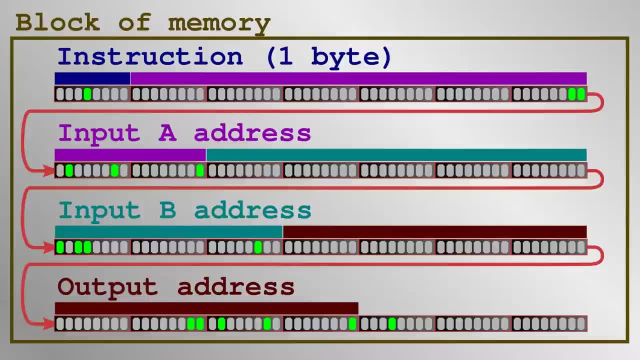 entire add instruction has one instruction byte and 24 bytes of addresses, 25 in total. On the other hand, if the instruction is to copy a number, it just needs to be followed by the origin and destination addresses. meaning the whole thing takes 17 bytes in total. The trick is that each 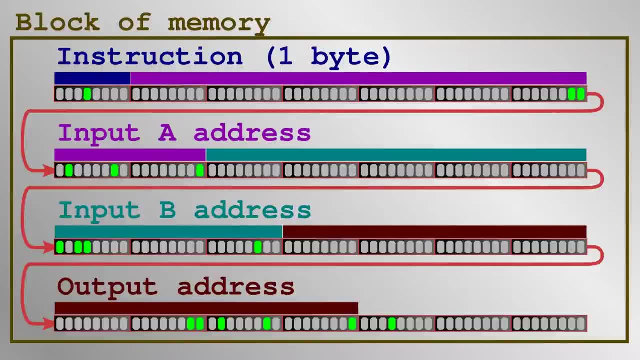 type of instruction always takes up a set number of bytes and, crucially, the next instruction immediately follows on after the previous one. So when the computer encounters the add instruction, not only does it carry it out, but it knows that the next instruction is precisely 25 bytes along. 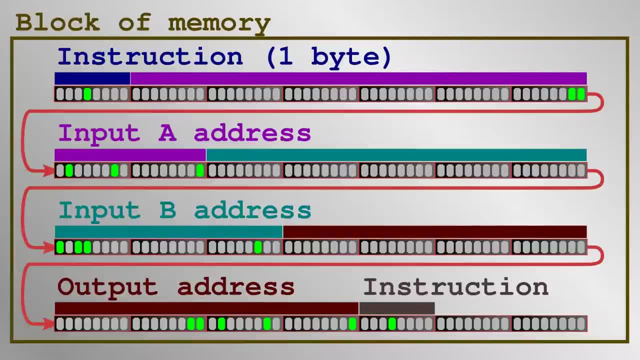 The add instruction is the one that starts with zero, the one at the very start of memory as an instruction and thereafter goes from instruction to instruction. Conversely, if there has been an error and the next instruction is not where it's supposed to be, tough luck, the computer will. 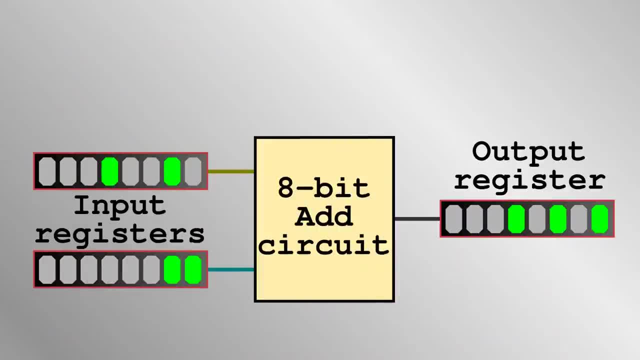 probably crash. How does the computer actually carry out an add instruction? The number from the first address is loaded into one input register and the second address into another input register. The add circuit is enabled and it does the addition Then, after a sufficient number of clock. 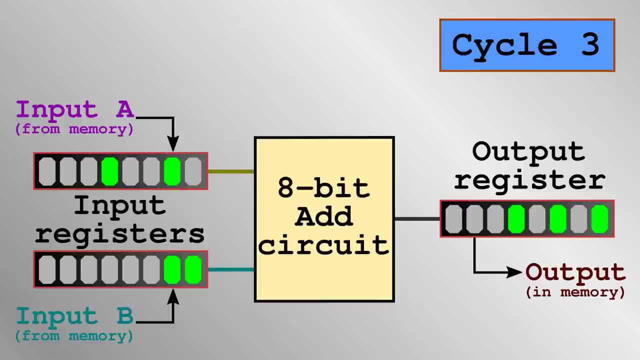 cycles. the result can be written from the add function, the output register, to the required address in memory. What happens if the instruction is to add two 16-bit numbers together? The computer simply goes to the address of number a and instead of getting just one byte, it gets that byte and then one immediately after The same for number b and 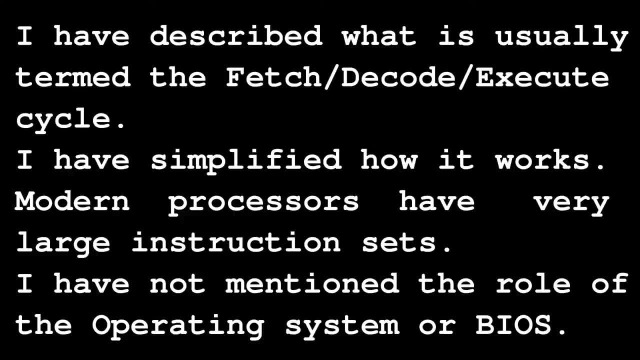 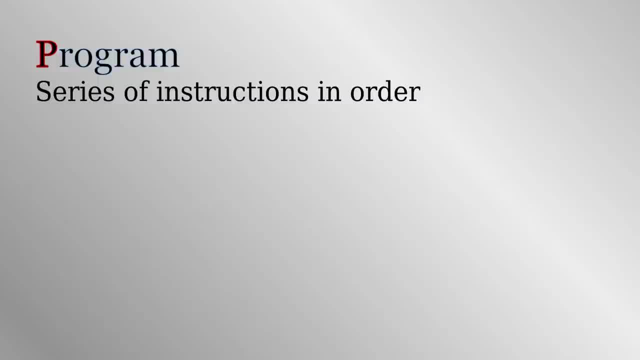 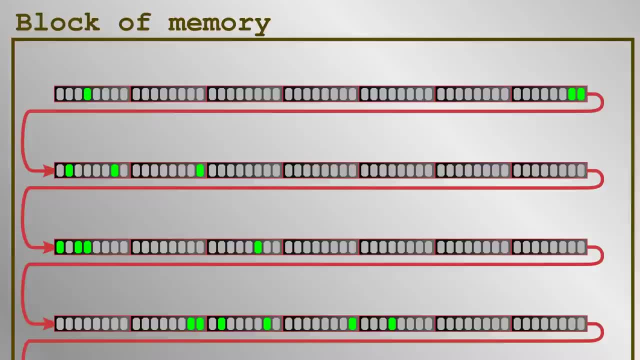 the result. c. A computer program is a collection of instructions and addresses to be done in order. The computer goes from instruction to instruction to make the program run. Let's look at a specific example, Part of the game- which is just a program after all- where the player has a wallet with coins in. 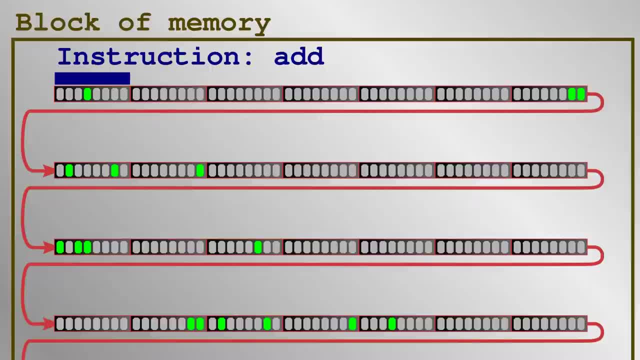 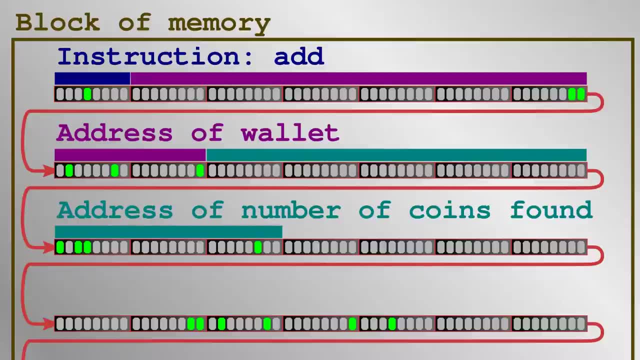 This is what the contents of memory might look like. Byte number zero is the instruction to add. Then come two addresses: The address of the wallet total and the number of coins the player has just found. The third address is the wallet, again After the addition. 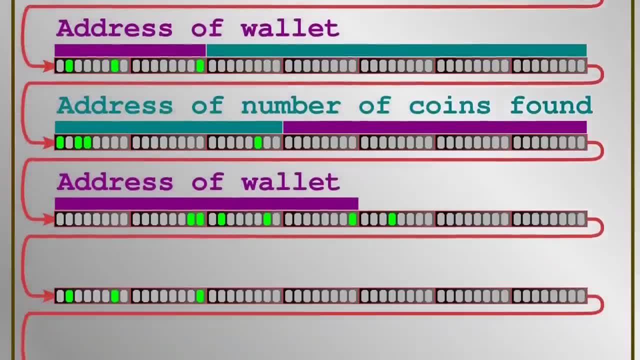 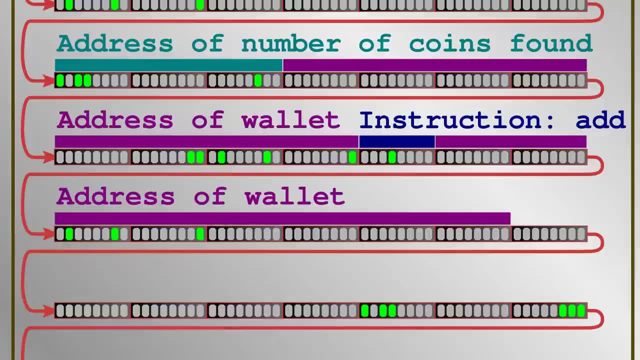 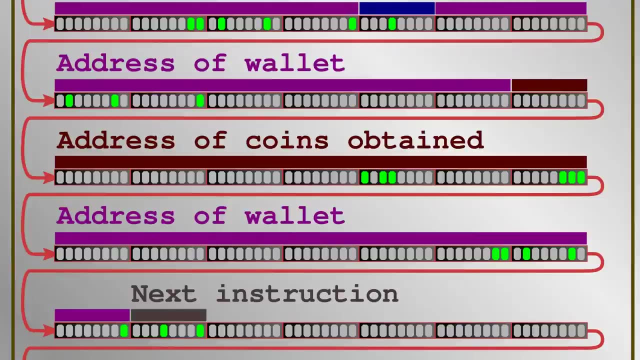 the wallet total will be overwritten, No matter what. the computer will now interpret byte number 25 in memory as an instruction. It is another add instruction And an amount of coins the player has made from selling items are the inputs. The wallet addresses the output again. The next instruction is 25 bytes further along at byte 49.. 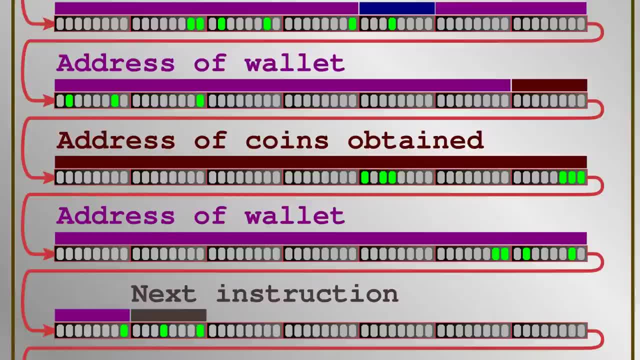 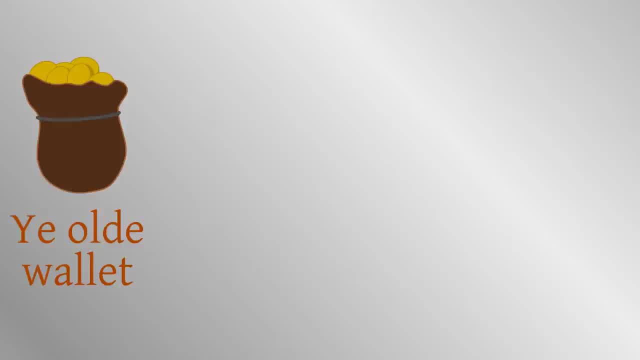 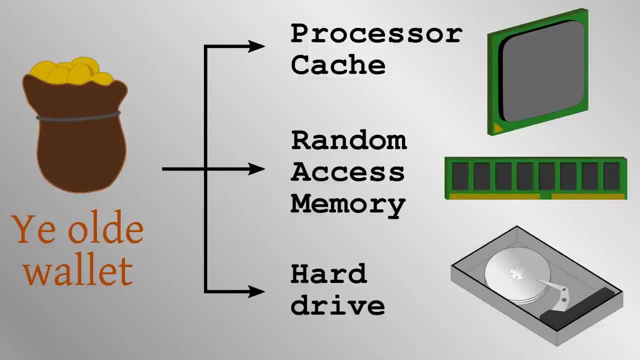 The program keeps going on with millions of other instructions required to make the game function. In this case, the wallet total is being used a lot, so it will probably be held long term in the processor's cache as well as the RAM. When the player saves the game, it will be written to a save file on the computer's hard disk. 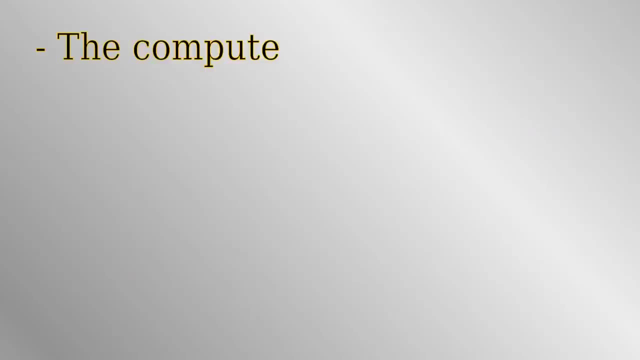 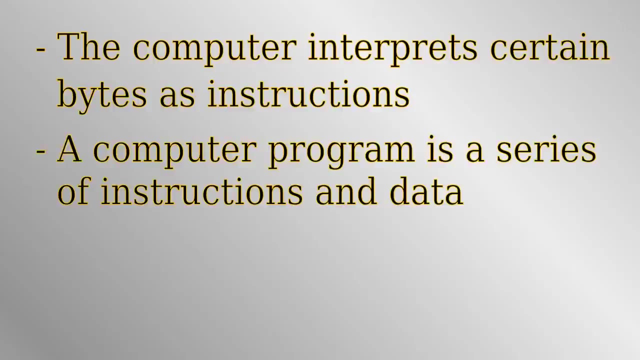 To summarize: the computer interprets certain bytes in memory as instructions for which operation to carry out. Computer programs are stored in memory. They are just large sequences of instructions, memory addresses and numbers. The computer goes from instruction to instruction like clockwork. 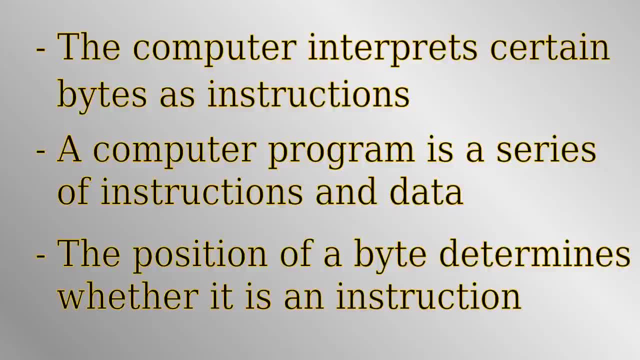 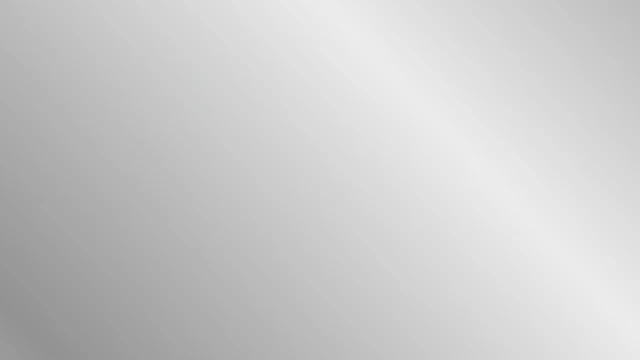 always knowing, based on the type of the current instruction, how far along the next one is. So far, we've looked at instructions which work in a linear manner: Copy a number, add two together, and so on. The program would always produce the same result. 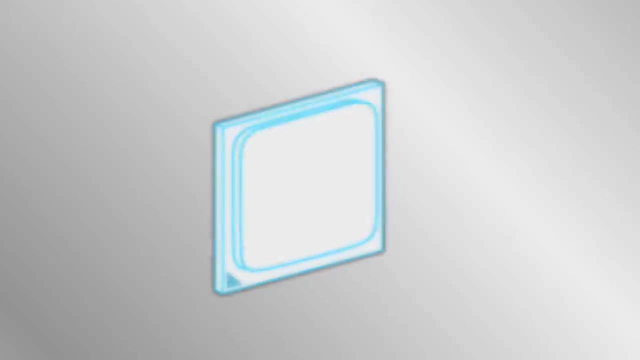 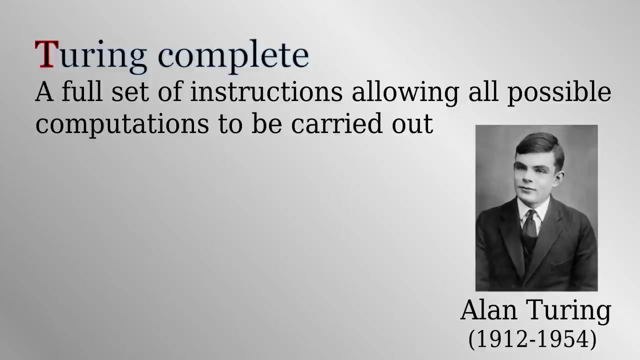 and eventually it would just get to the end of memory and stop. We need a few more instructions to make a computer what's known as Turing Complete. Being Turing Complete means that it can eventually carry out any possible computation: Load a web page, render a video game, and so on. 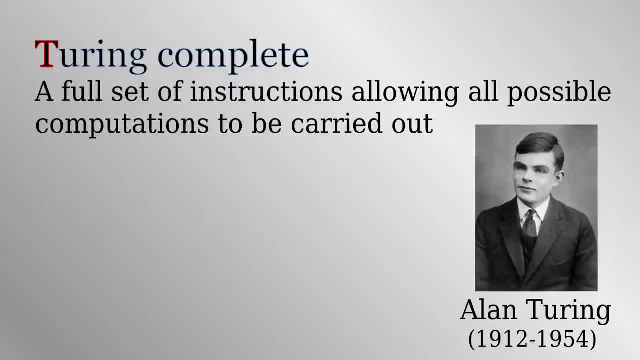 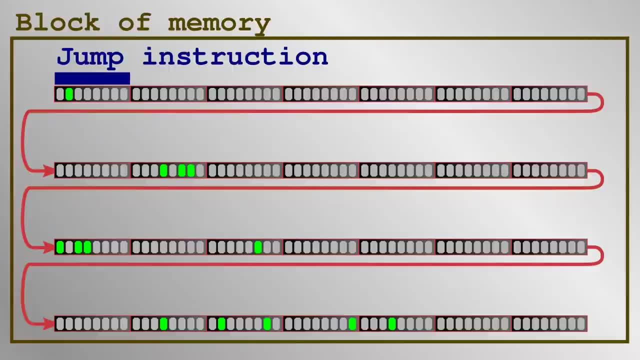 The only difference between two Turing Complete computers is how fast they are at doing it. The first type of instruction a computer needs is what's called a jump, or sometimes called a go-to. Following the instruction byte is a memory address, As the name suggests, instead of going directly to the next instruction in memory. 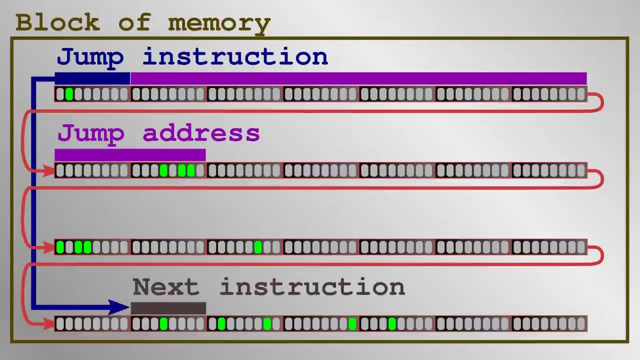 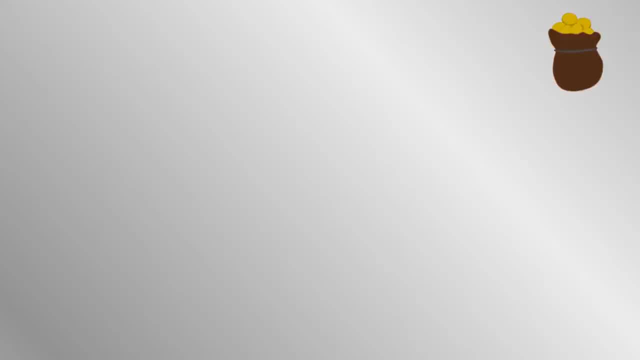 the program jumps to the specified memory address and carries out the instruction there. This means that the program can now do a loop. In our video game example, we have seen how instructions are used to add numbers of coins to a total kept in a wallet. 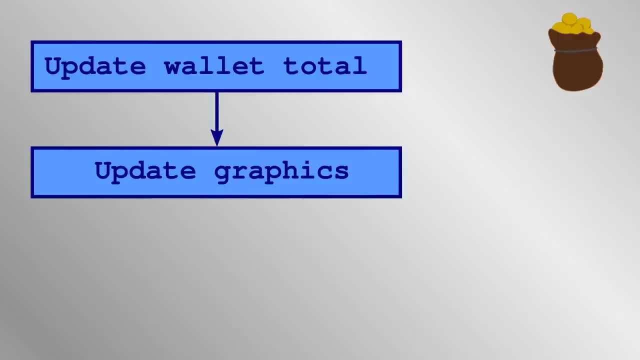 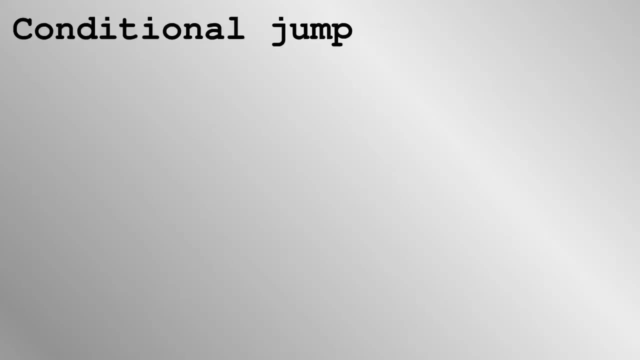 These instructions and all the others required to update the game world, render the graphics and so on, are followed by a jump instruction back to the start. This way, the game can keep running indefinitely. The other crucial type of instruction that a computer needs is a branching or conditional. 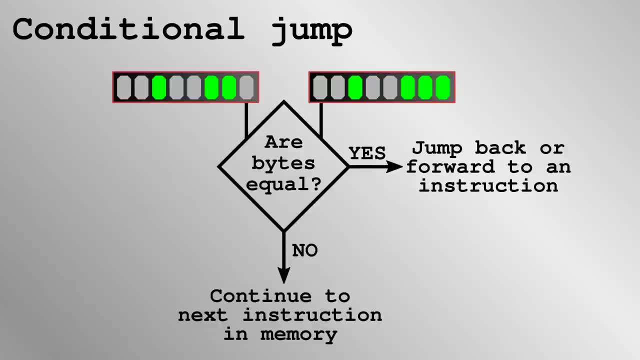 instruction If a given condition is met, for example, if two numbers are equal, then jump to a particular address. We have already seen how a comparison can be implemented with logic gates. Adding such logic makes a jump conditional, allowing different sets of instructions to be executed. 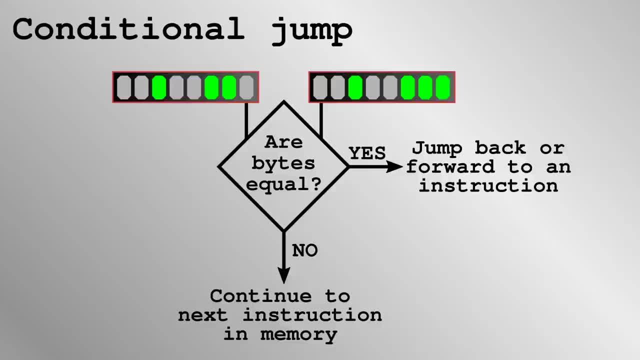 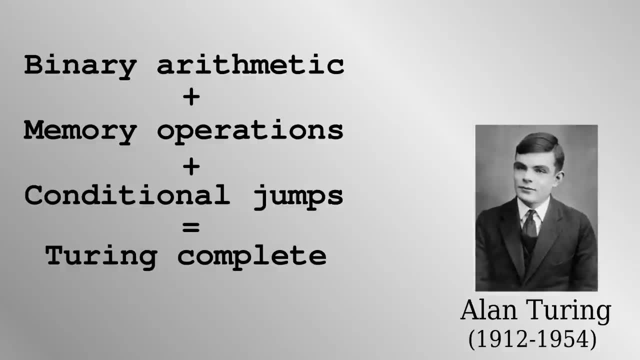 based on calculations performed so far or inputs to the computer such as a keyboard or mouse. With conditional jumps, the computer is Turing complete. Given enough time, it can do any calculation. At this point it's worth mentioning how a real program might actually be written. 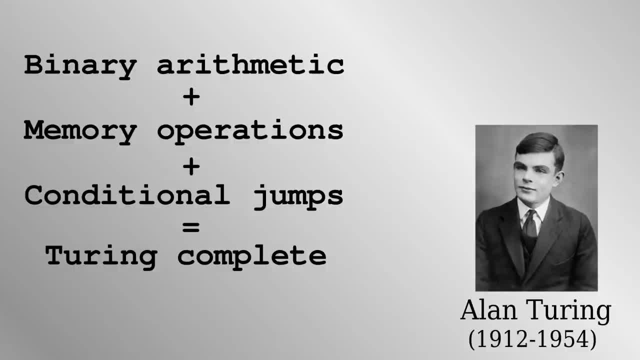 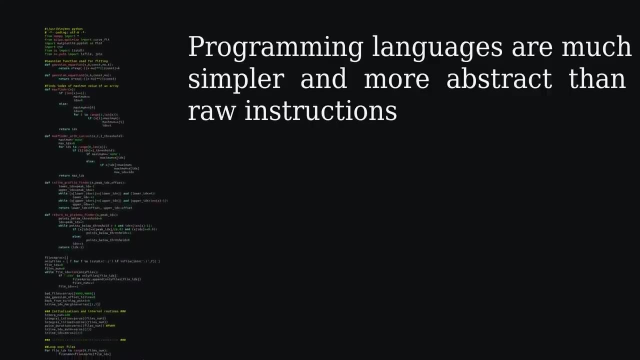 If you thought that things were quite confusing so far, you're not wrong: Remembering which instruction does what, which memory addresses have what data stored in them, where jumps go, and so on. This is all hard to keep track of. Programmers typically work with what are referred to as high-level programming languages. 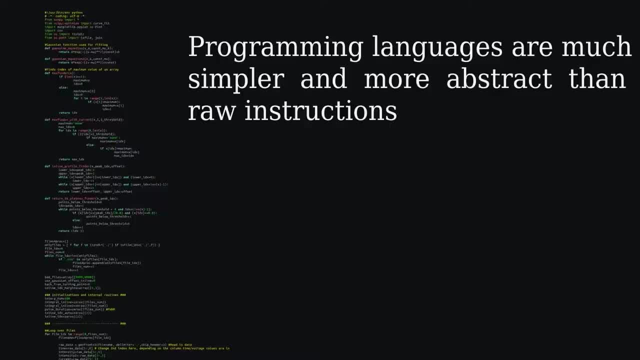 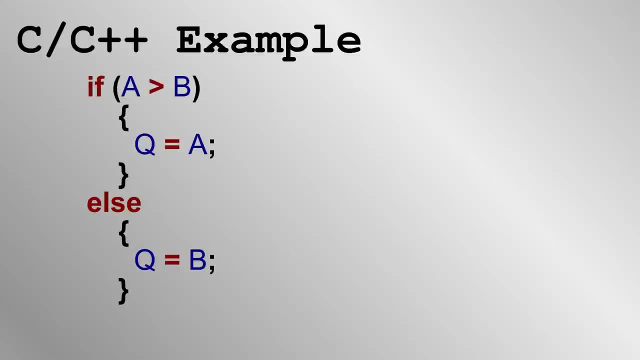 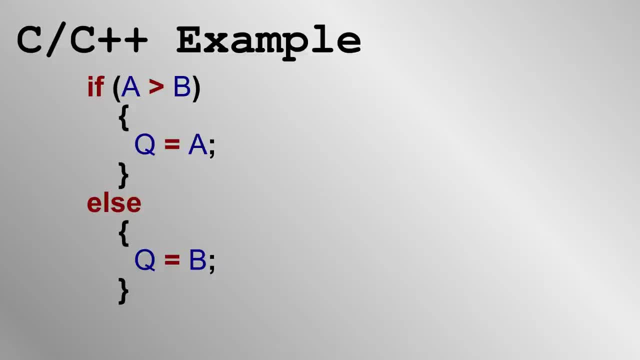 Otherwise, when B is greater or lower than B, set Q to be A. Otherwise, when B is greater or equal to A, set Q to be B. In other words, the number Q will end up with whichever number is larger out of A or B. 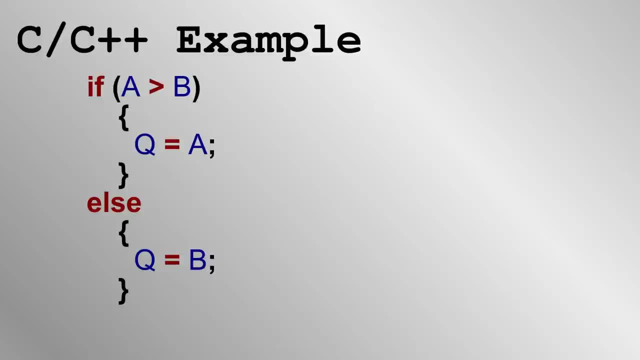 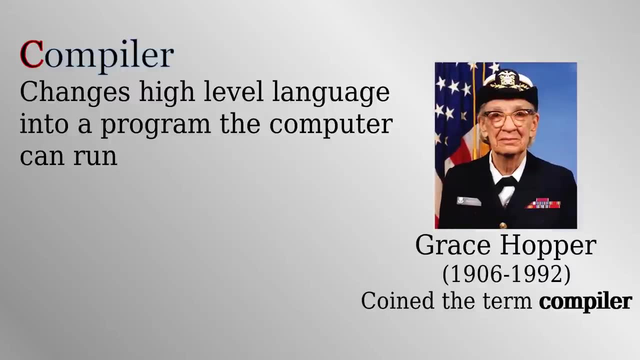 This is easy to understand for the programmer and anyone who tries to read it. A program called a compiler will take this code and arrange it into the correct set of instructions, sort out where the variables are stored in memory, where to jump- do we need to use 16-bit or 32-bit numbers? and so on. 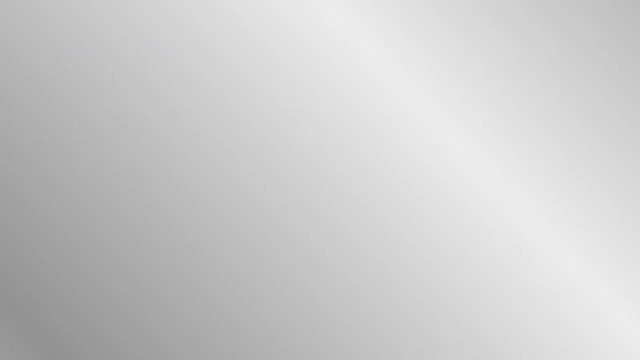 This is what's referred to as compiling the code. There are many aspects of programming language. There are many aspects of programming language which simplify the job of the programmer, But one of the most important is the idea of a function or method. In mathematics, the square root is a function which takes a number and returns another. 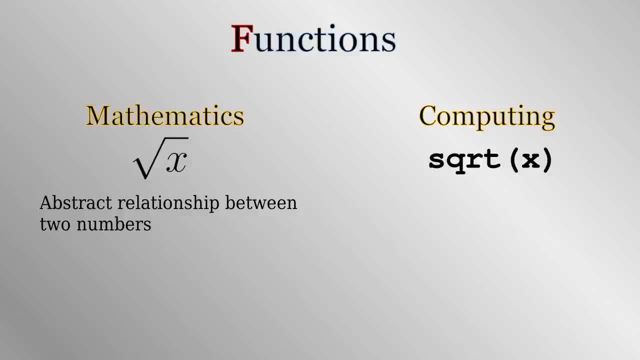 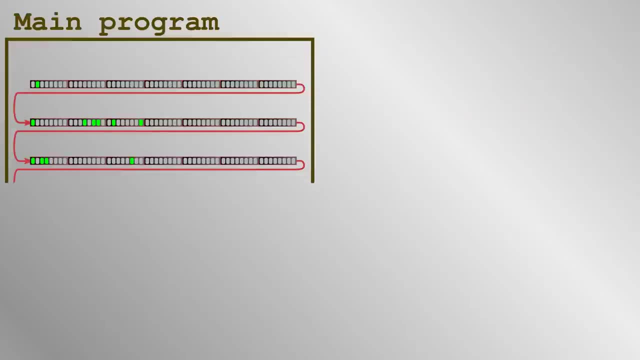 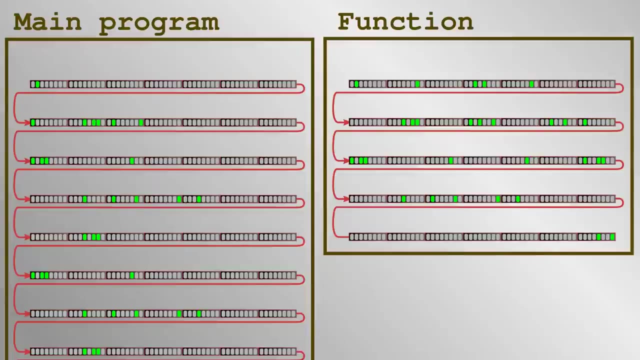 Certainly there are implementations of the square root function in computer code, but there are also more arbitrary functions, and methods such as for fetching emails and so on Say that a program needs to evaluate the square root of different numbers repeatedly. The instructions which comprise the square root function need only be stored in memory once. 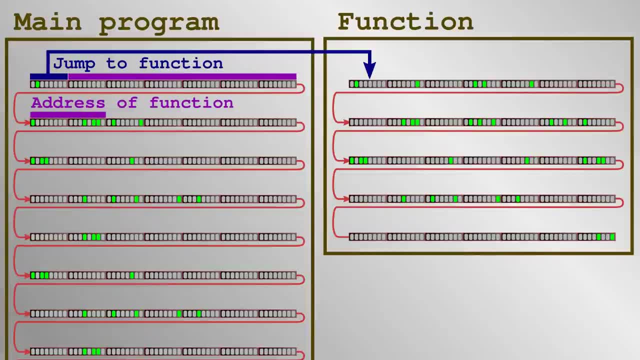 Whenever the function is stored in memory, it needs to be stored in memory once. Whenever the function needs to be used or called, the computer will jump to the function's location in memory, carry out the instructions and jump back with the result to the place in the program where it left off. 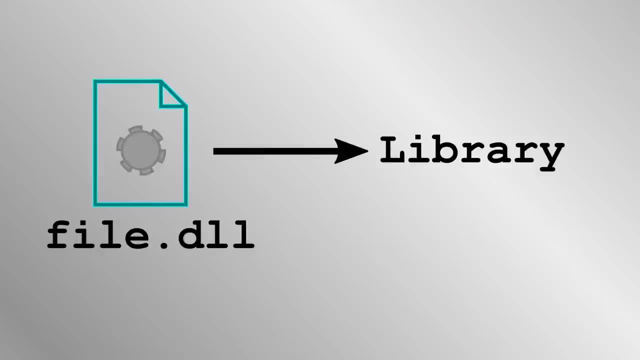 Functions and methods can be compiled into libraries so that programmers across time and space can share useful code that they've written. If you've ever seen a DLL file on Windows, that's what that is: Once a function or method has been written efficiently. 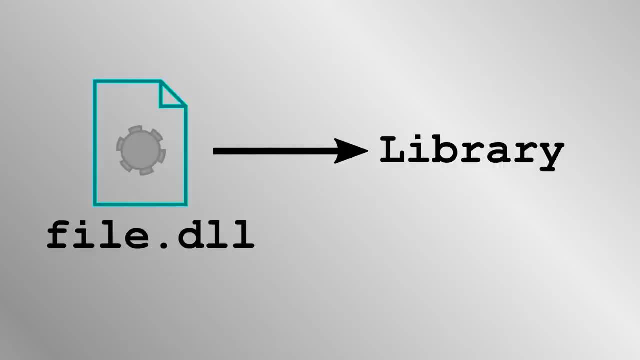 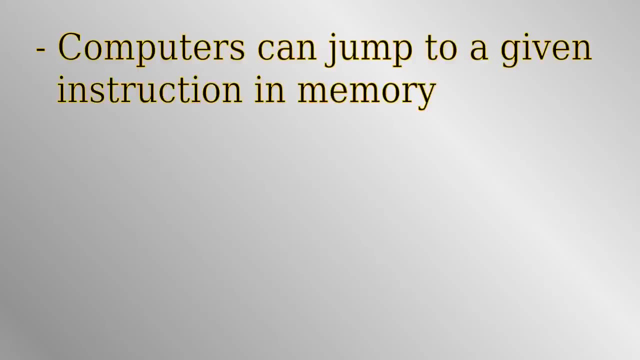 other programmers can use it without needing to spend much time on it. To summarize, computers have an instruction to jump to a memory address and carry out whatever instruction is there. This allows loops within programs. Some jumps only happen when a condition is met. 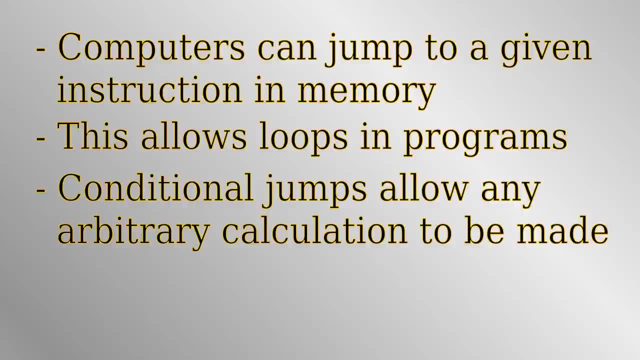 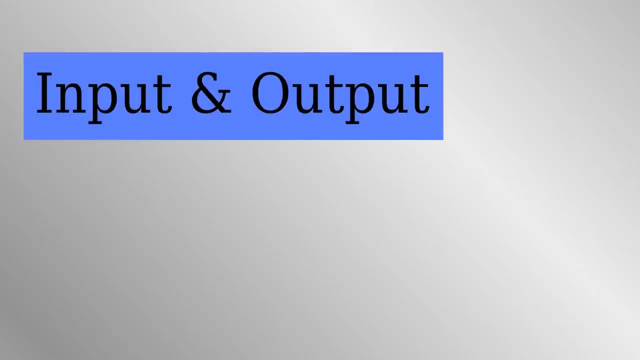 Any computer that is capable of such jumps can carry out any computation, as long as it has enough memory and time to do so. Chances are you're watching this video on some sort of display. There are many technologies that can be used to do this. 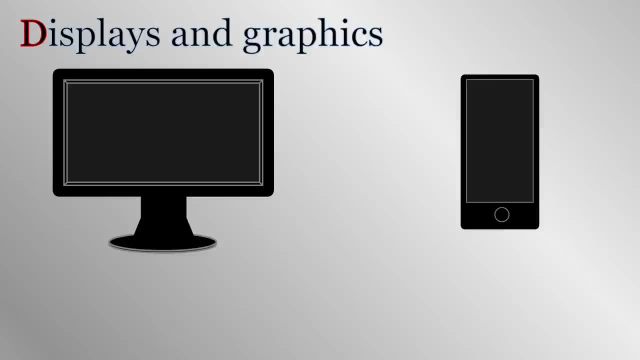 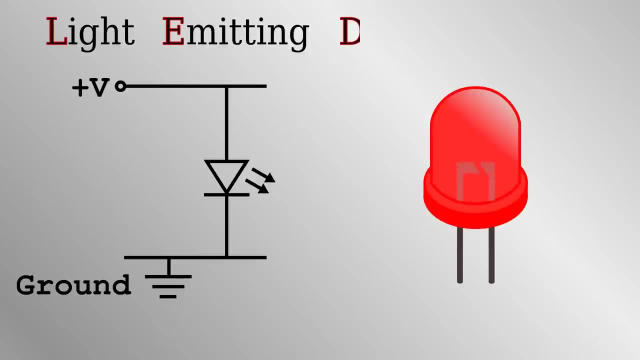 There are many technologies, past and present, which have been used for computer monitors, so I will speak in generalities. Light bulbs, like at the start of the video, are too large, but light emitting diodes or LEDs are smaller and more efficient. The higher the voltage across an LED, the brighter it is. 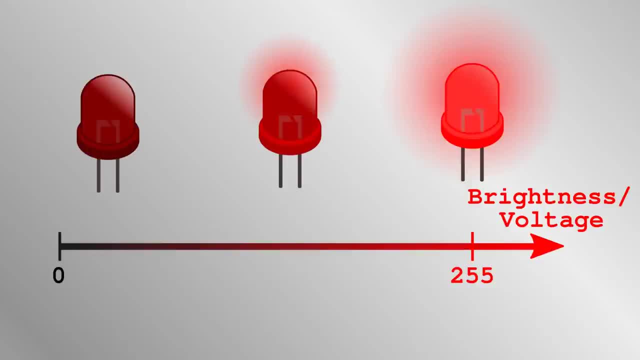 A display is capable of electronically changing the voltage across each of its LEDs, and therefore their brightness, according to data from the computer. Since computers handle numbers in bytes, in other words groups of 8 bits, it makes sense to have the brightness go up on a scale from 0 to 255,. 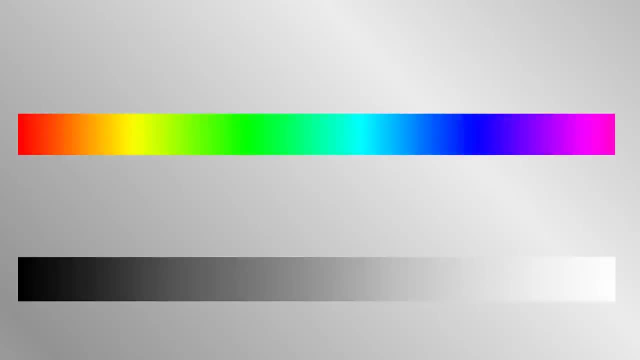 the largest value a byte can take. The human eye has cells sensitive to red, green and blue light. By using a set of three LEDs- red, green and blue- varying the relative brightness of each one, the human eye can be tricked into perceiving the full spectrum of light. 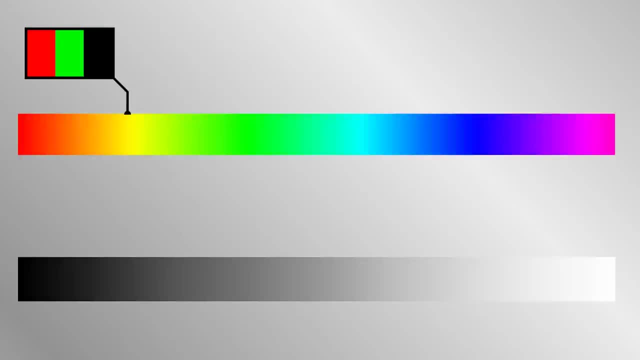 A mix of red and green gives yellows and browns, red and blue, gives pinks. all three colours at full brightness give white, and at partial brightness they give yellows and browns. At partial brightness they give white, and at partial brightness they give yellows and browns. 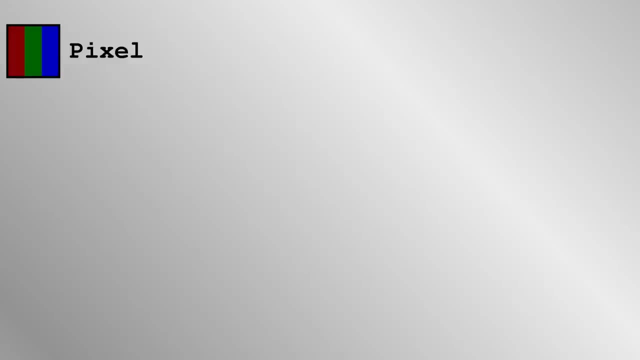 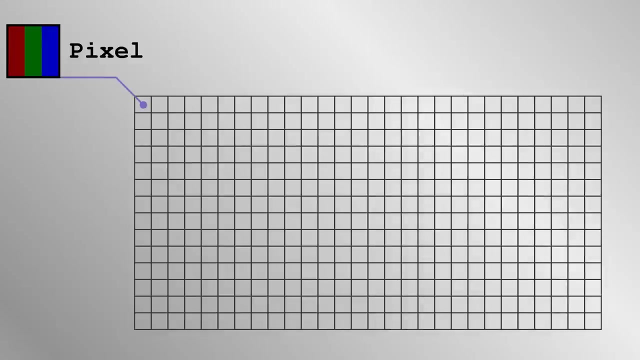 At partial brightness, they give grey and so on. A little spot composed of three colours like this, no matter what technology is used, is called a pixel. A display has pixels arranged in rows and columns to form a two-dimensional grid. For example, this video at maximum resolution is 1920 pixels in width by 1080 pixels in height. 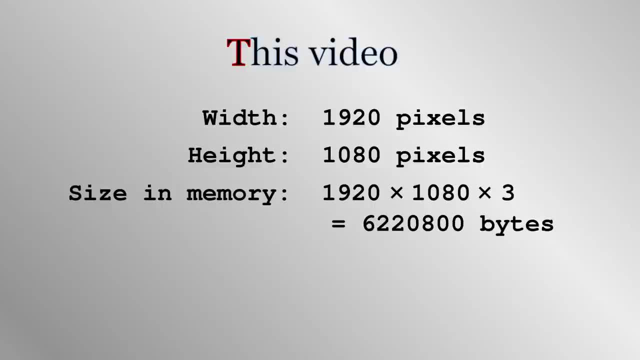 The number of bytes it takes to fill a display in memory is 3 times the width, times the height. In simplest terms, the computer must update this many bytes in memory 30 or 60 times per second and send the result to the display. 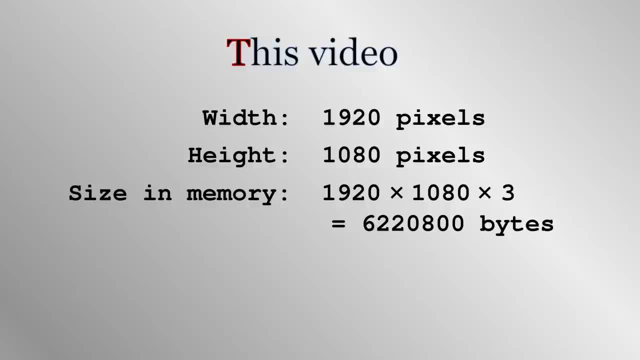 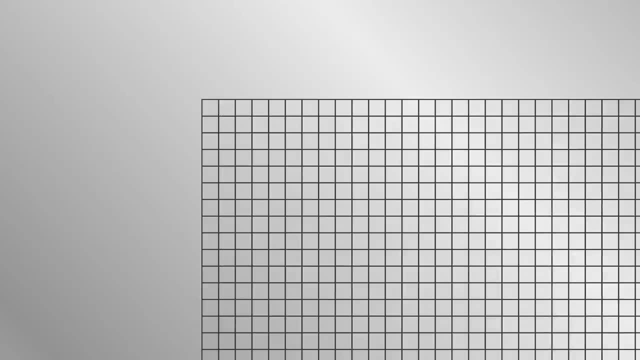 So, for example, if you full screen this video in its maximum resolution, each frame would take up this many bytes in memory, While displaying graphics and images may seem like a purely artistic undertaking, and in some sense it is in actual fact. for a computer, it is nothing more than. 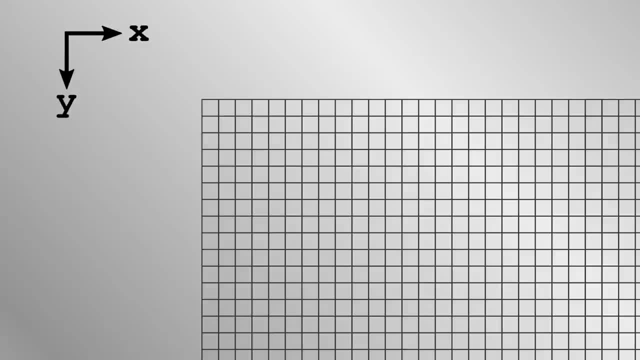 gate logic and instructions we have seen so far. Each pixel has a horizontal or x coordinate and a vertical or y coordinate which corresponds to its position in memory. For example, let's say your display is exactly 1000 pixels wide and you start with the top left pixel. 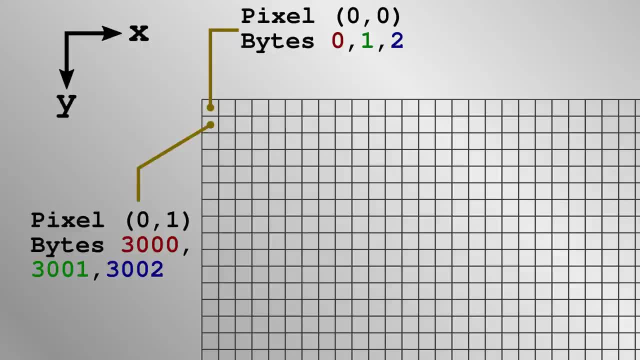 If you move forward 3000 bytes in memory, or the equivalent of 1000 pixels, you will go off the end of the top row and onto the left pixel of the second row. There are many algorithms or long lists of instructions to draw windows. 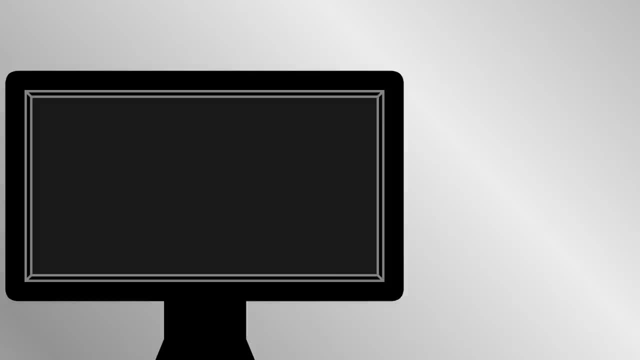 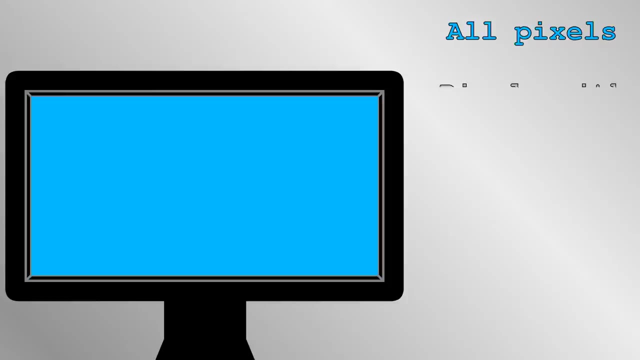 buttons, text and computer graphics, using this kind of arithmetic and manipulating bytes in memory To display a simple desktop environment. a loop fills every pixel with a background color by repeatedly copying the sequence of three bytes that uniquely defines the color. The taskbar is drawn by looping over only rows of pixels with specific y coordinates. 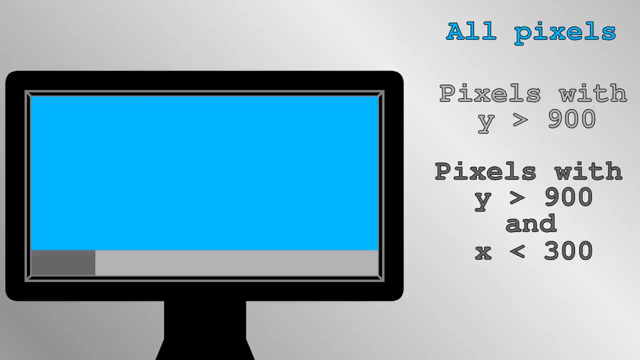 A start button is created by filling a rectangle with a given range of x and y coordinates with another color. Text is added on top by copying predetermined patterns of pixels for each letter or through some other algorithm. To display a window, it's necessary to know its specific width and height. 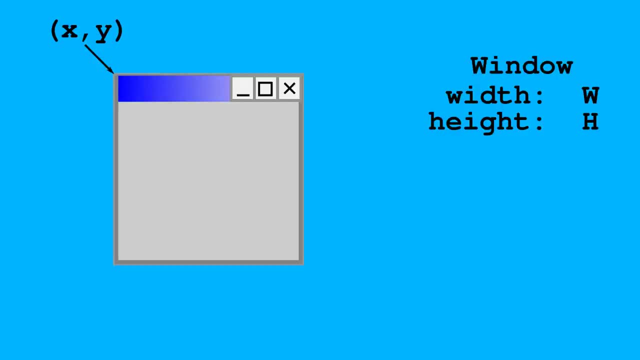 and the current position of its top left pixel. Adding the x value of the left pixel and the width by simple arithmetic gives the rightmost edge pixel. A title bar can then be drawn along with a border text and so on. If the user moves or resizes the window, all of this arithmetic has to be redone and the window redrawn. 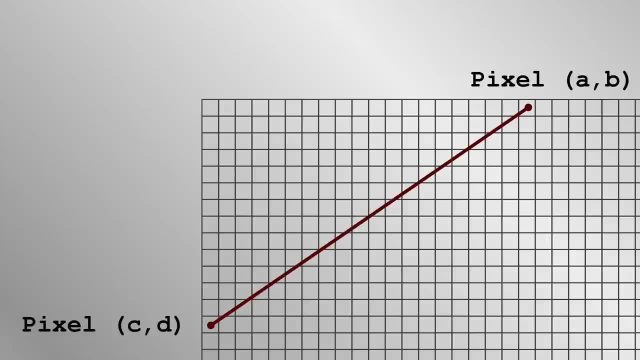 The simplest computer graphic involves drawing a line between two points, both with their own set of coordinates x- y. The Bresenham algorithm involves a loop which draws just such a line by following a straight x- y curve familiar from school mathematics. 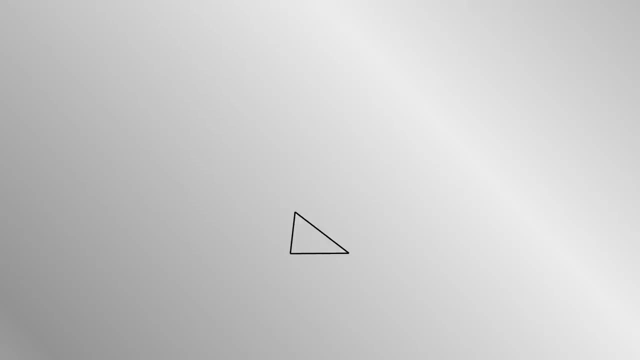 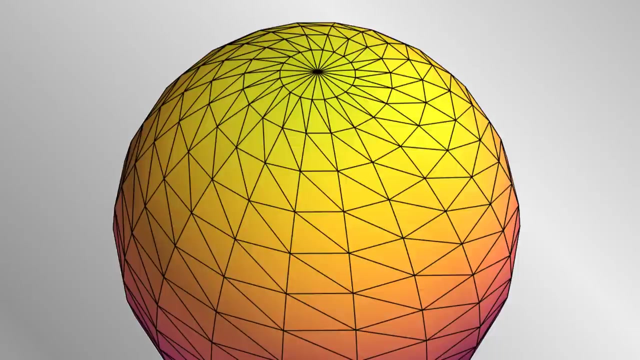 Draw three lines and you have a triangle which can be filled with textures, illuminated by simulated light sources and combined with thousands of others to make a 3D shape. No matter how complicated, it all comes down to addition, multiplication and jump instructions compiled into functions. 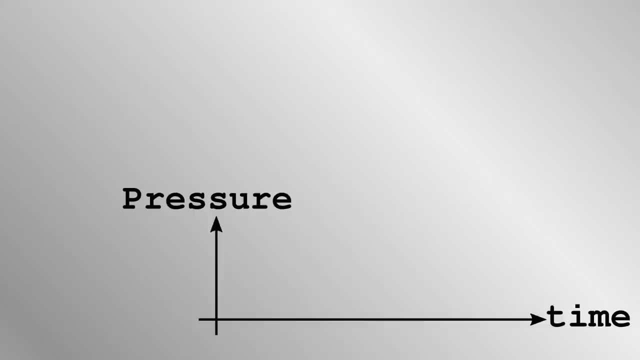 Sound is the other major form of output from a computer. Sounds are waves of high and low pressure moving through the air. Speakers and headphones produce sounds by moving a membrane back and forth. There is a permanent magnet attached to the membrane inside a fixed conducting coil. 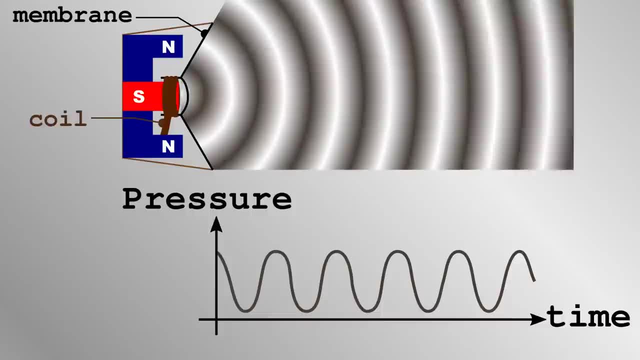 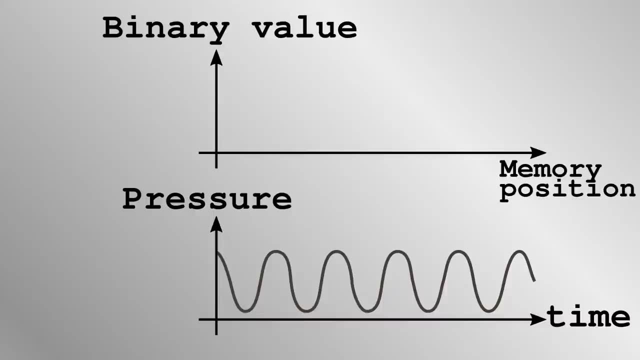 An oscillating current through the coil pulls the magnet in and out, making the membrane oscillate and creating a sound. The computer breaks up time into short steps and specifies the current at every step in time by sending a binary number to a sound card. 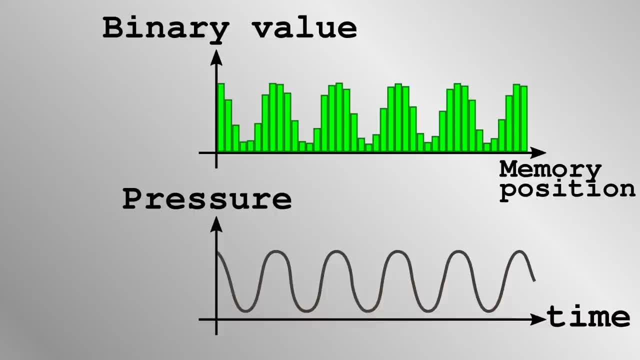 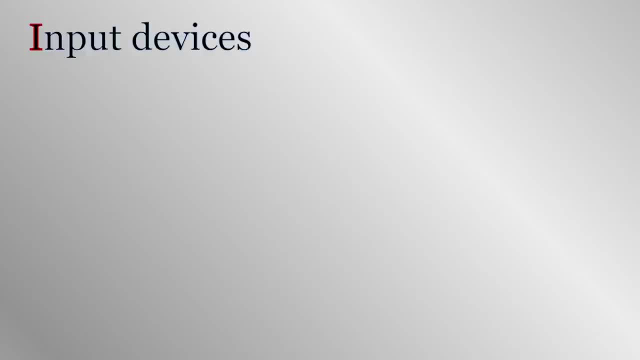 Electronics turn the digital binary values into their appropriate coordinates. A microphone works in exactly the opposite way. There are many input devices out there, but the way a computer deals with inputs is usually the same. The inputs leave so-called messages in memory, which are groups of bytes of preset length. 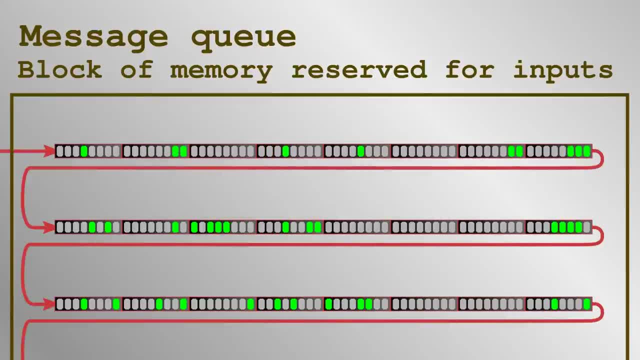 identifying the device and what exactly the input consists of. For example, a message queue may have in it three messages of eight bytes each. When decoded, the first one states that the A key has been pressed down. The second states that the mouse has moved 30 pixels to the right. 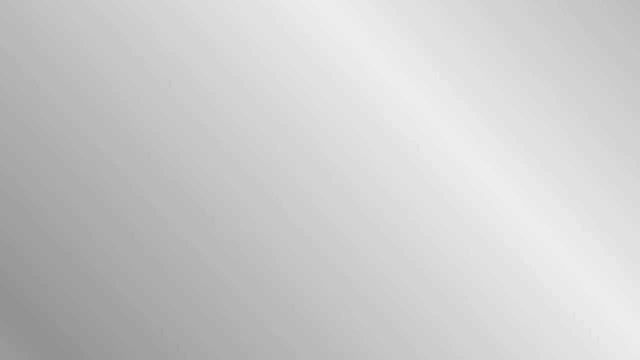 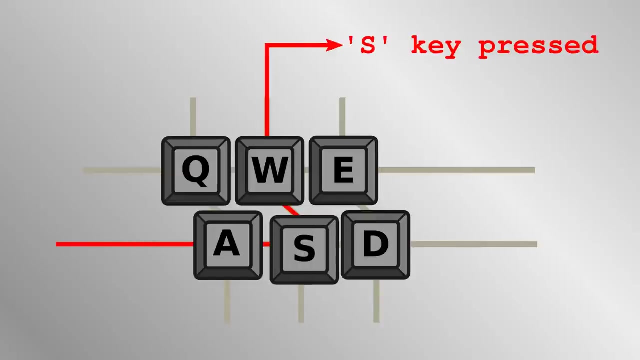 and the third, that the Shift key has been released On a keyboard. the keys are arranged into a grid. When a key is pressed, it makes an electrical contact between a horizontal and vertical row, allowing the precise key to be identified Between the keyboard and the computer's motherboard. 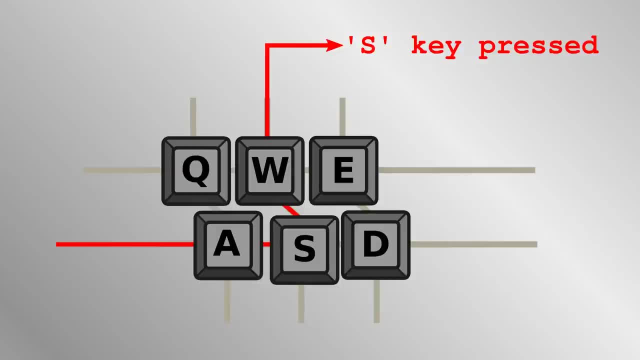 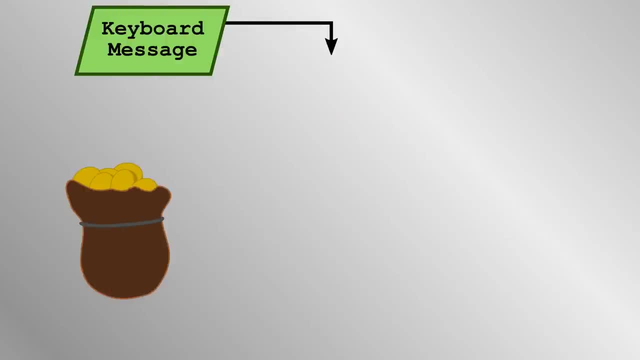 the message announcing when a key is pressed down or released is relayed to computer memory, allowing the computer to act on it. In our video game example, imagine that the B button is the key, the C button is used to buy things and the S button is used to sell. 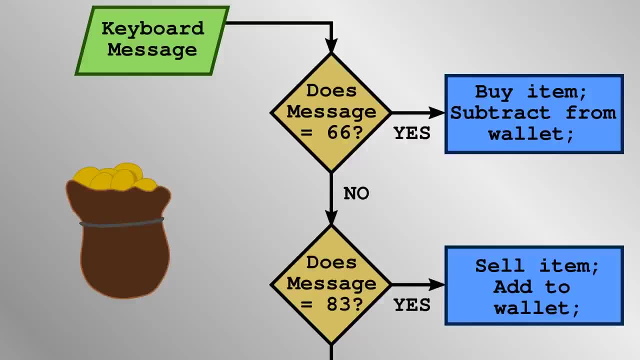 In Windows, these key presses have corresponding decimal numbers, 66 and 83, respectively. In terms of instructions, the game would have conditional jumps based on the value of the last keystroke. If the keystroke value is 66, then a computer would jump to a set of instructions corresponding to buy. 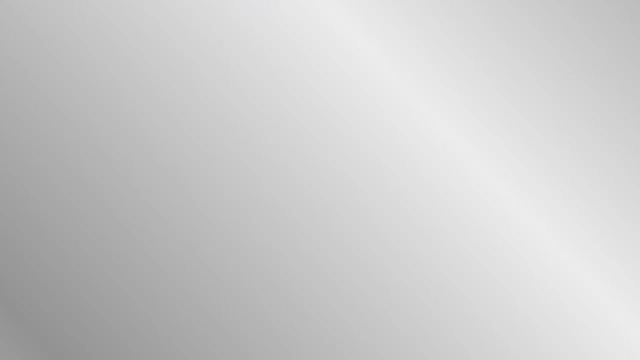 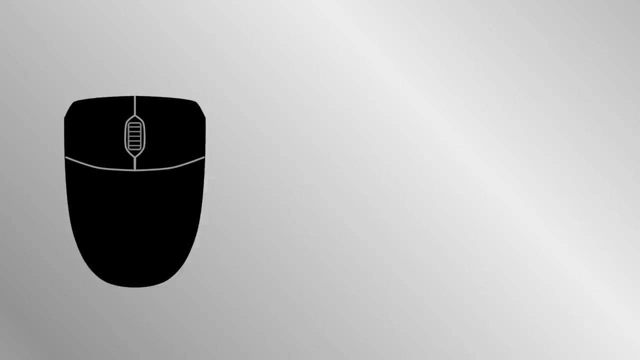 If 83, it would jump to instructions corresponding to sell. A computer mouse tracks how far left or right and up or down along a flat surface and also which buttons have been pressed. A program, typically the computer's operating system. 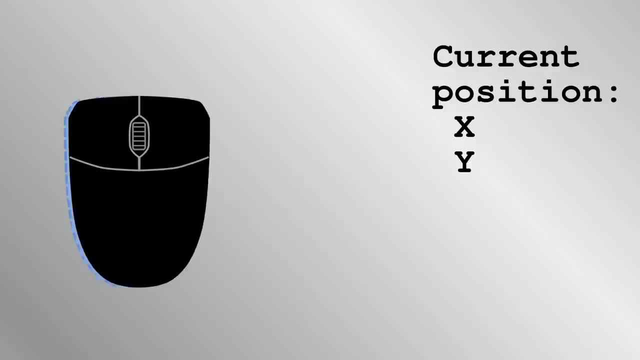 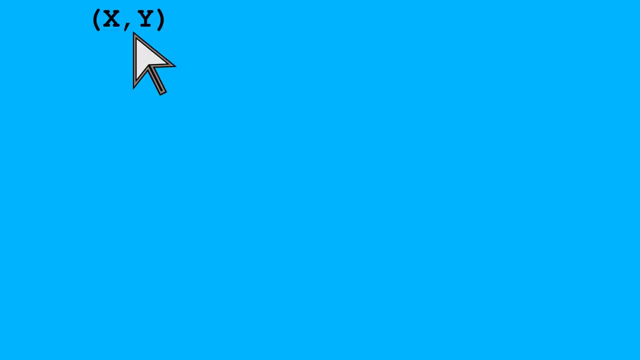 keeps track of the X and Y pixel coordinates of the mouse by adding or subtracting any changes in position received from the mouse. Say that a window with a button is currently active. when a user presses down the left mouse button, The program will check the X coordinate of the mouse cursor against the dimensions of the button.